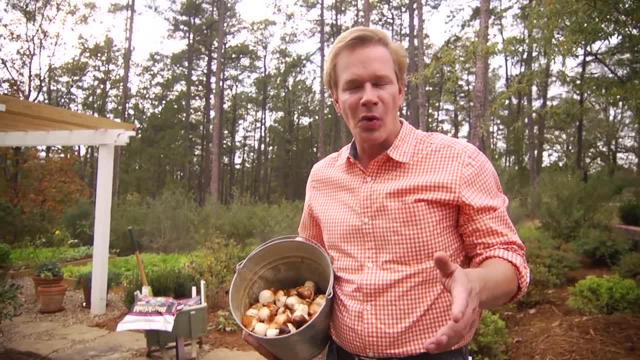 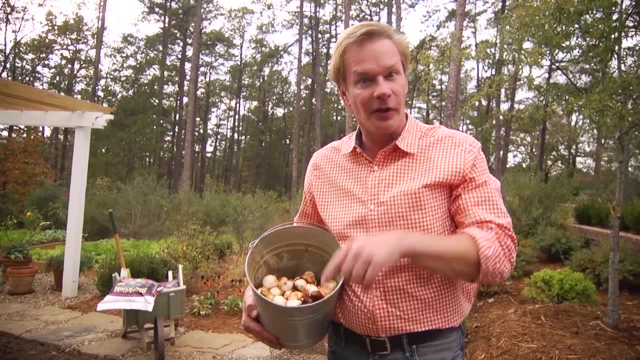 Are you one of those people who drive around in neighborhoods in the spring and go: oh my gosh, I love all those beautiful tulips, I want some. Well, if you want some, you have to plant them in the fall. Now's the time to plant them. Let me show you. 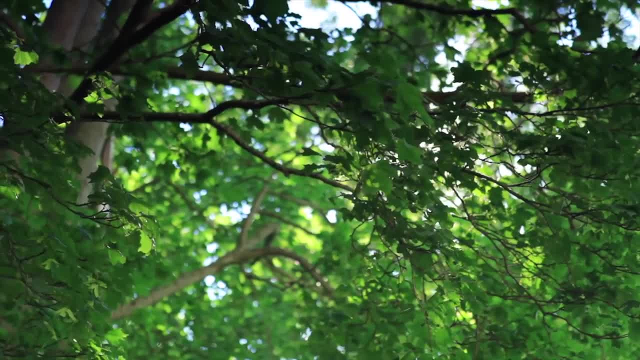 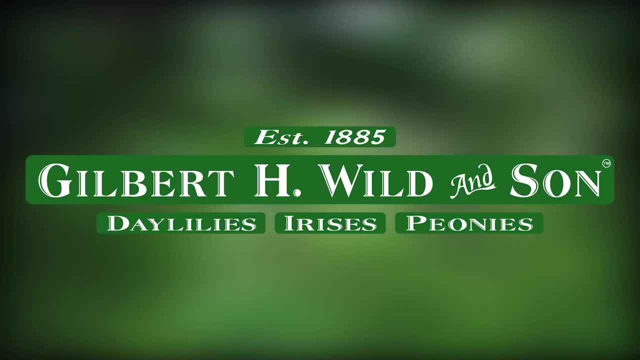 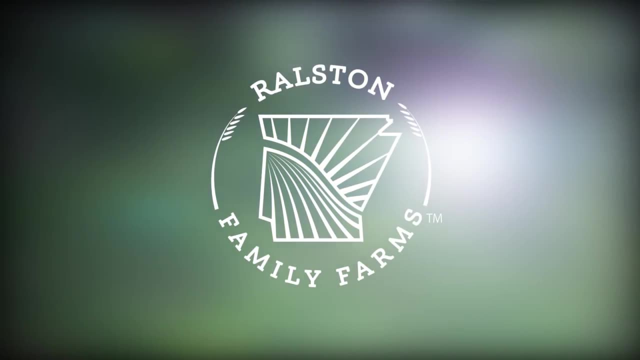 Before we go any further, I'd like to thank our sponsors. The garden tours are made possible by Gilbert H Wild and Son, who've been growing beautiful perennials since 1885.. Ralston Family Farms: a farm family producing delicious rice for your table. 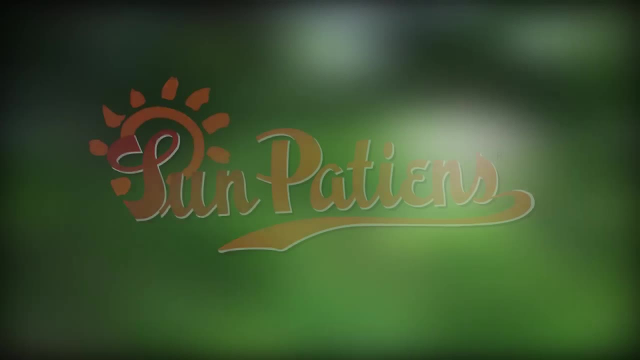 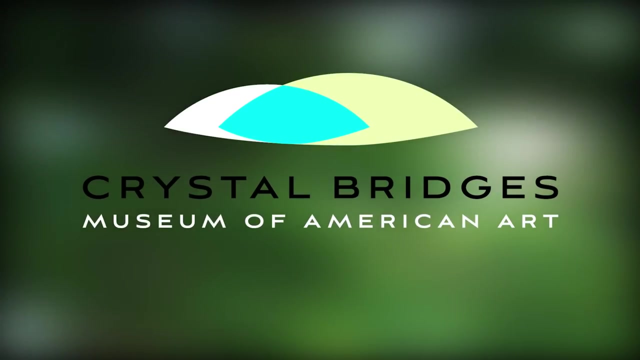 First Community Bank, whose heart is in the community, as well as Sun Patience, Super Cow, Petunias and Dragon's Breath, Celosia And Crystal Bridges Museum of American Art. Check out my website to learn more about the brands we love. 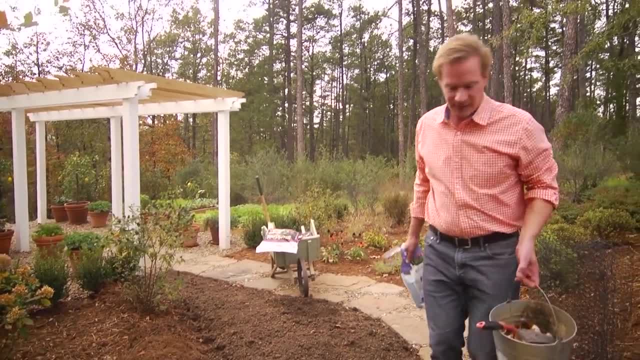 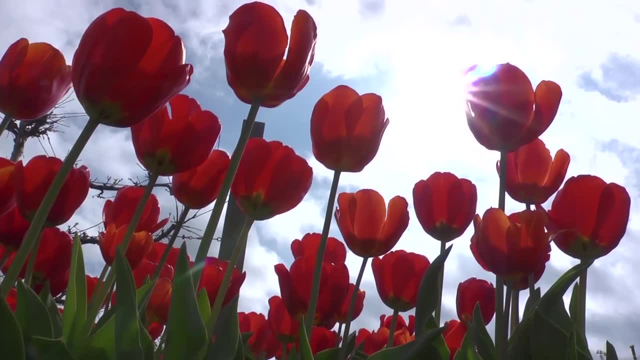 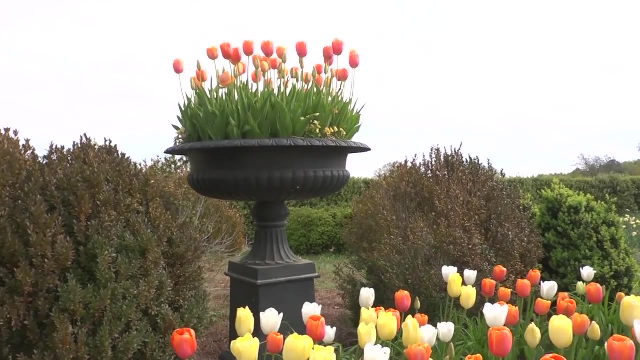 Who doesn't love spring flowering bulbs? Well, I certainly do. Tulips are one of my all-time favorites. If you love tulips and you have a favorite color, I'd love to know what you love- Mine. well, I'm crazy about these apricot-colored ones. I plant them everywhere And I'm planting some. 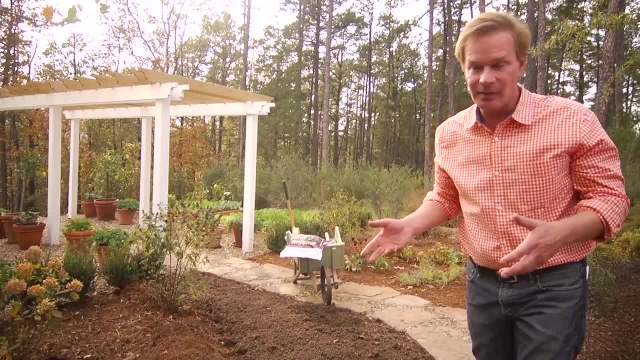 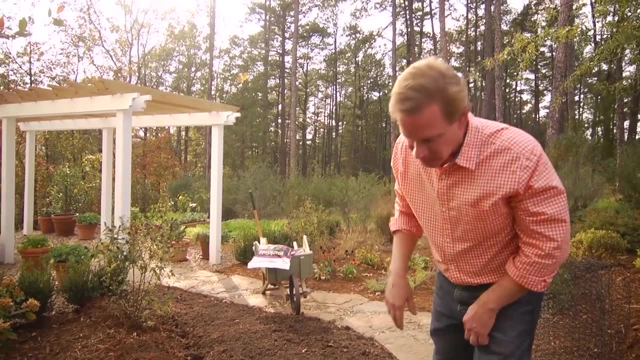 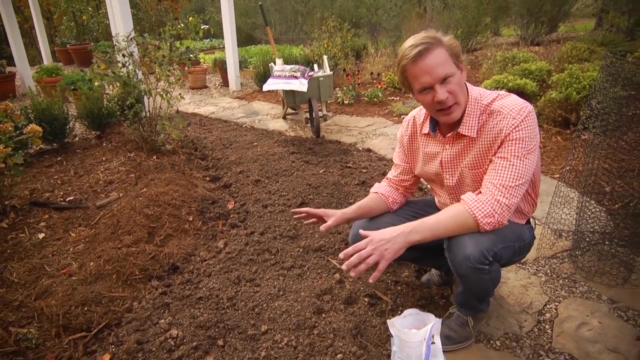 called Minton, And this is the time of year to do it. It's fall. If you want those spring blooms in March and April and May, you gotta plant them now. So what I've done here is I've prepared a bed Now. this isn't gonna be all bulbs. We're gonna overplant it later with some things, But 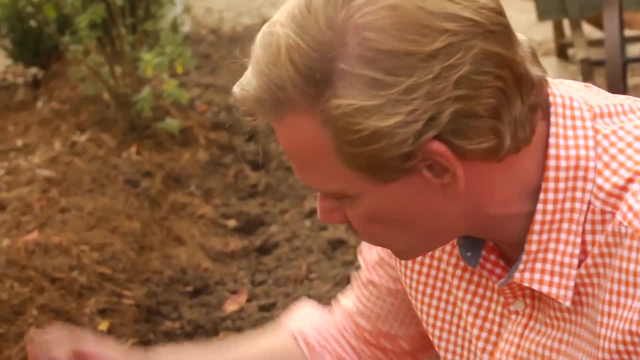 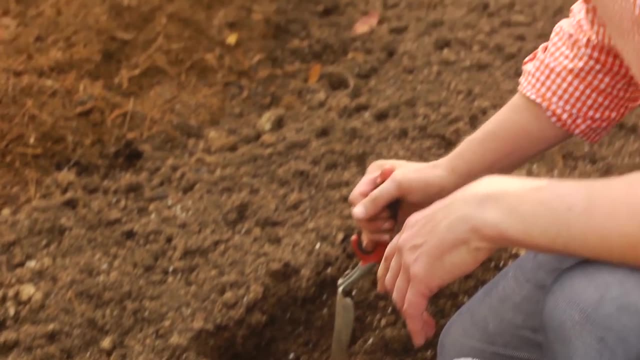 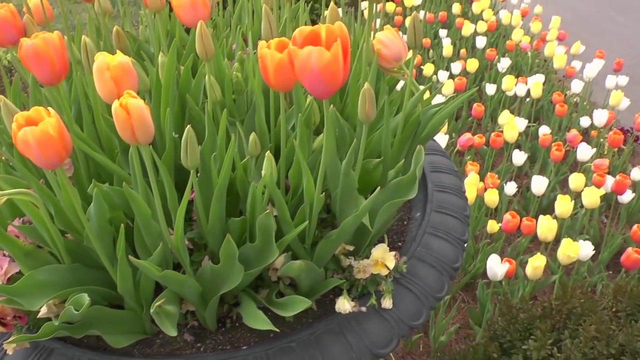 what I like to do is work the soil up, And you can see that this soil is really deep, So I can drive this trowel into the ground almost nine inches, And that's what you want. When I plant bulbs, I want a lot of visual impact. I tend to plant a lot of the same variety. 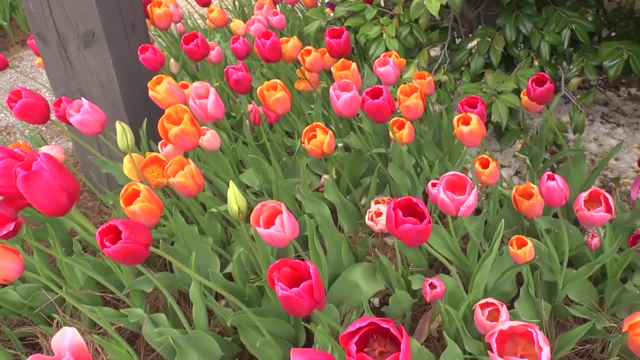 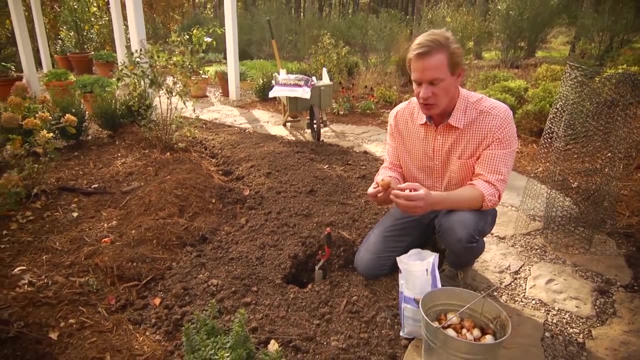 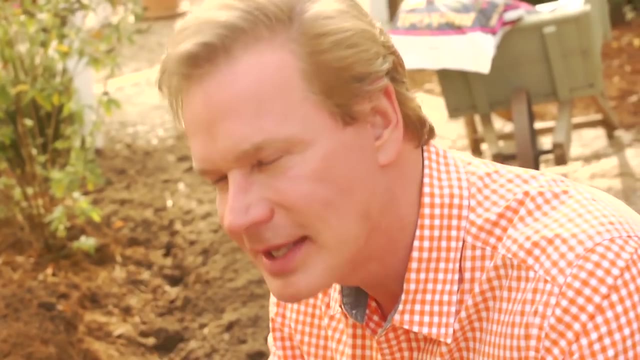 or varieties that work together in terms of color. I also wanna think of when they bloom. You may not know this, but depending on the variety of tulip you choose, you can get varieties that bloom early in the season, midway in the season and late in the season. So when you're thinking, 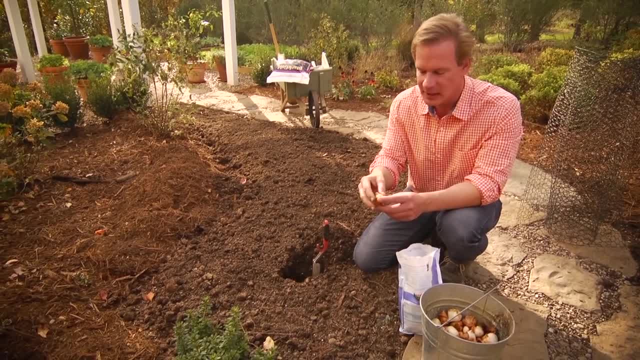 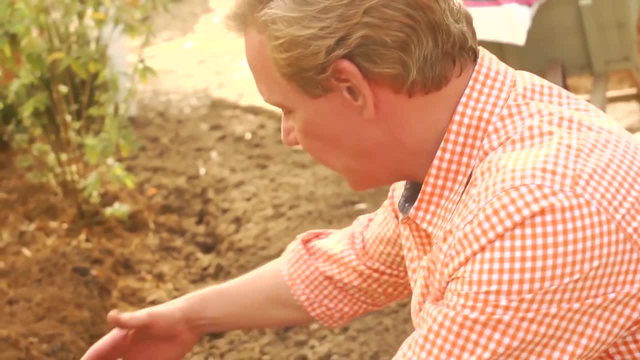 about planting some tulips this fall – and I hope you will – think about that, because you can have a continuous bloom. In this case, since I'm so crazy about Minton, I'm gonna do a big grouping of them here, a grouping of them there and then one down there, And then I'm gonna fill in with a. 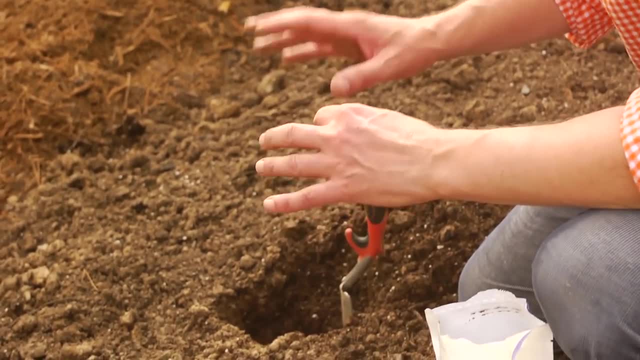 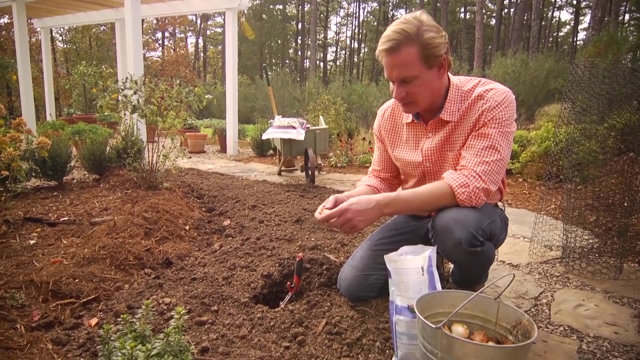 lot of spring-blooming annuals over them And I'm telling you, next spring this flower bed will be a knockout. So let's get back to planting these bulbs. I'm gonna go ahead and plant them here. When I plant the bulbs, I like to plant them about 25 to a group- a nice drift- And I plant them. 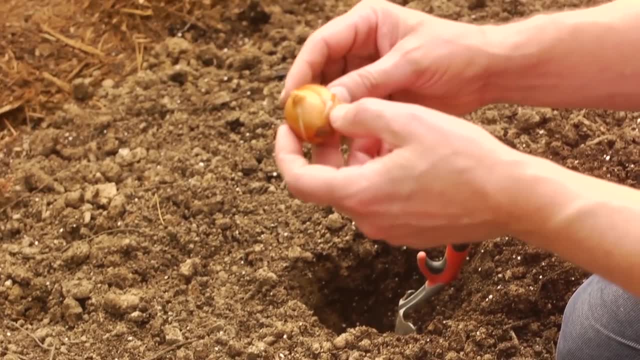 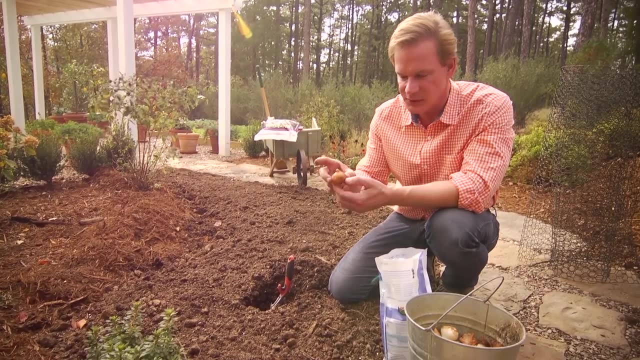 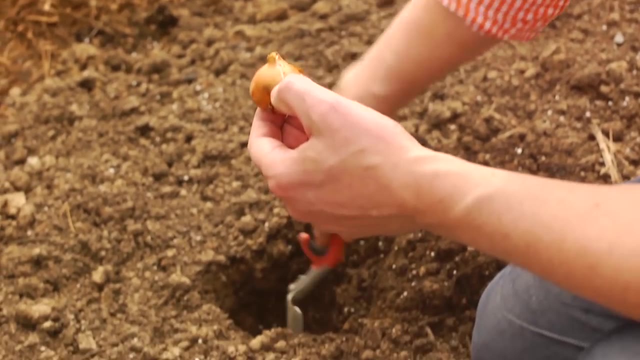 you know, about eight inches apart, And one of the rules for depth is to plant the bulb three times. You wanna cover the bulb three times its width, So if it's this wide – one, two, three – you'd want it about that deep, And so I've dug a hole about that deep here. 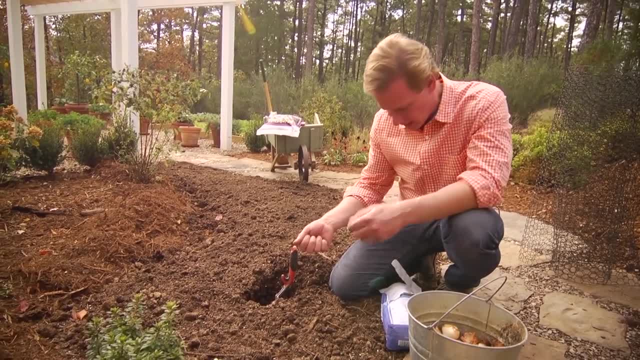 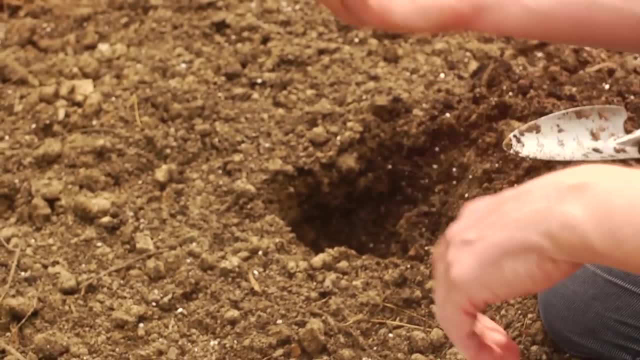 You just take a little fertilizer – I like to use an organic fertilizer for bulbs, specifically blended for it – about a tablespoon in there, And I work it around a little bit And then I drop the bulb in. You want the flat end or the basal plate end. 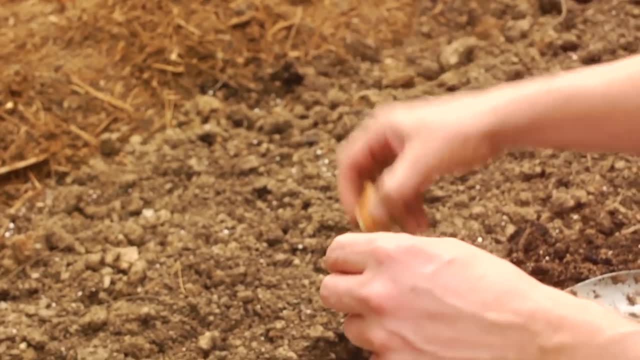 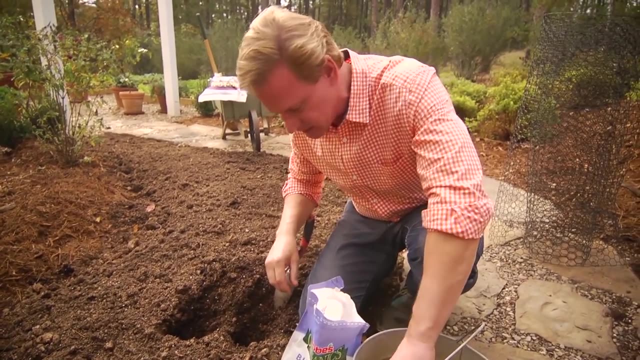 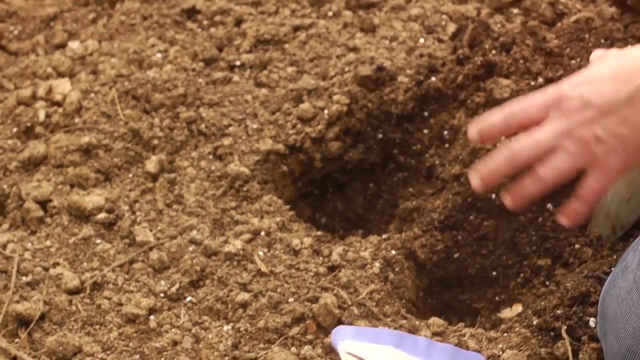 toward the soil like that, And what I like to do is go along and plant them so I can see them. So this one, I'll come in and I'll put this one next to this one so I can see exactly where they are. You get the idea: Put a little fertilizer in there, drop it in, Then I'll work my way around. 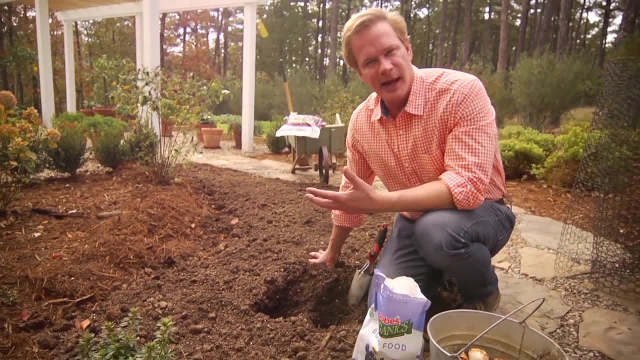 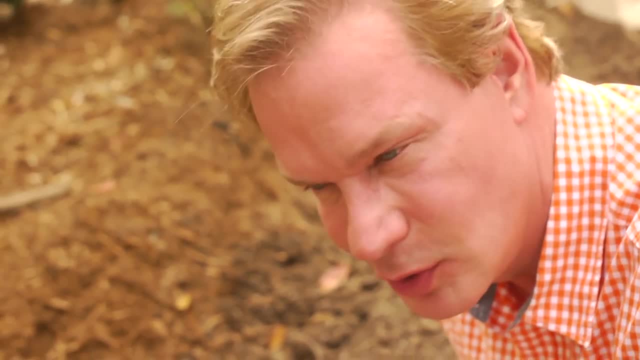 and I'll have this entire bed planted. Then I can decide whether I need to protect them, Because I know a lot of you have asked me questions about how do you protect your tulip bulbs from squirrels. Well, one of the best things to do is once you get the bed planted. 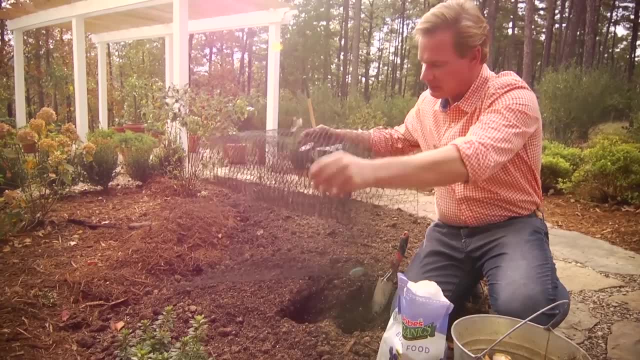 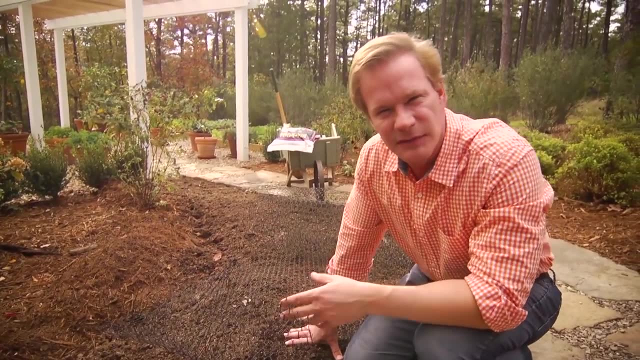 you can take some chicken wire – and this is coated with a little black plastic so you don't see it – and you can just roll this out over the top of the bed and just leave it there, Cover it with leaves, cover it with mulch, whatever you want. This will keep those little 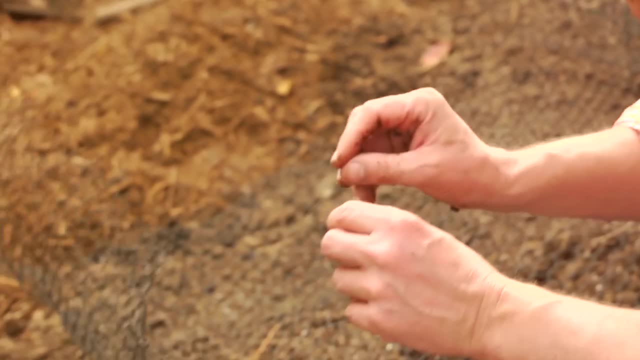 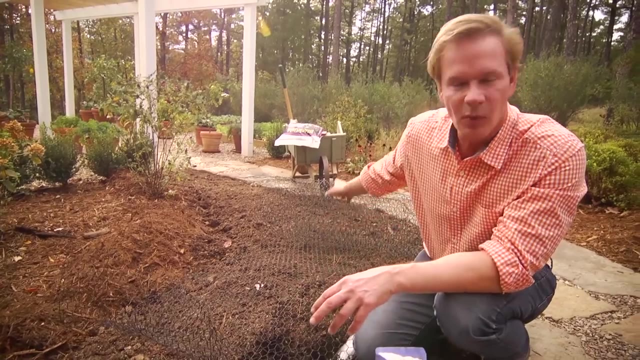 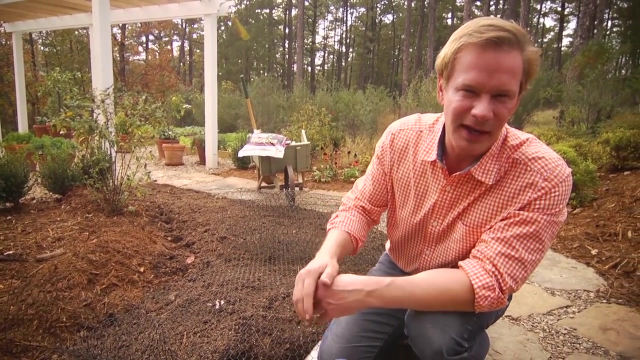 squirrels from digging up your tulip bulbs. Then, when winter is over and when you just begin to see the tips of those little bulbs pushing up, you can take the chicken wire off, put the mulch back around it. The bulbs will come up. At that point the squirrels don't really care, because the bulb is already rooted in, It's no longer a bulb, It's a full-grown plant And your bulbs will come up and bloom beautifully. This is a trick that's really worked well for me over the years. So when those temperatures are up, you can take the chicken wire and you can take the mulch and 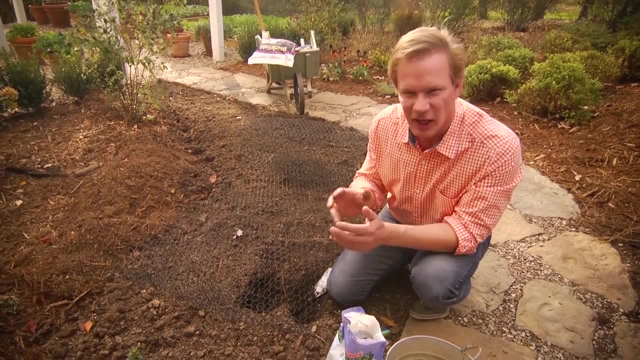 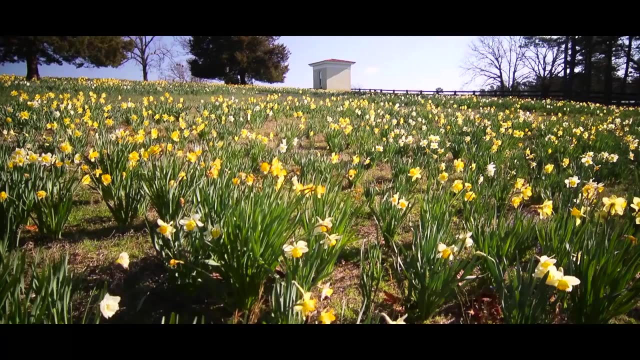 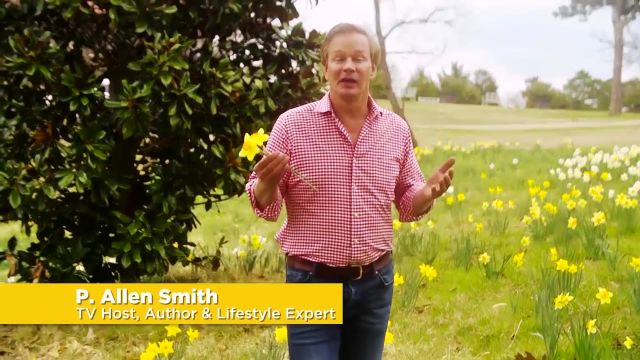 leave it there And when those temperatures begin to cool, make sure you go to the garden center and get lots of bulbs and get them planted. You'll be glad you did in the spring. Who doesn't love daffodils? What's there not to love? They're so. 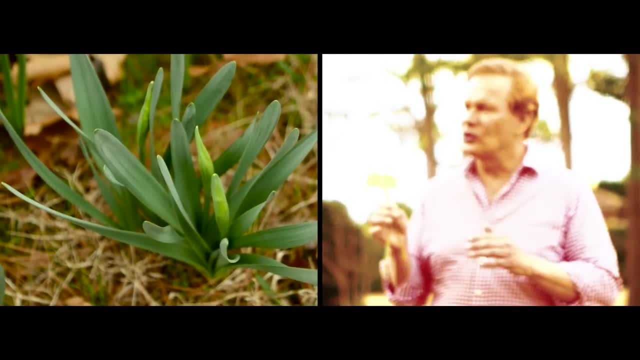 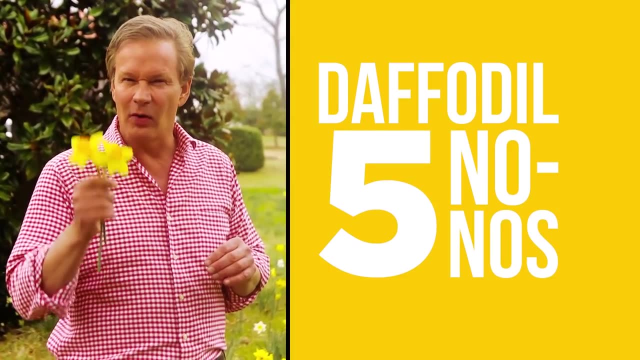 beautiful and reliable, But you may have trouble getting your daffodils to bloom. So what I want to do is I want to point out the five things that keep daffodils from flowering year after year. Number one: daffodils need to be planted in the sun. 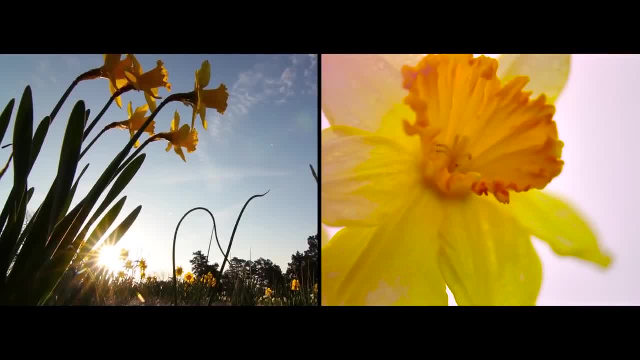 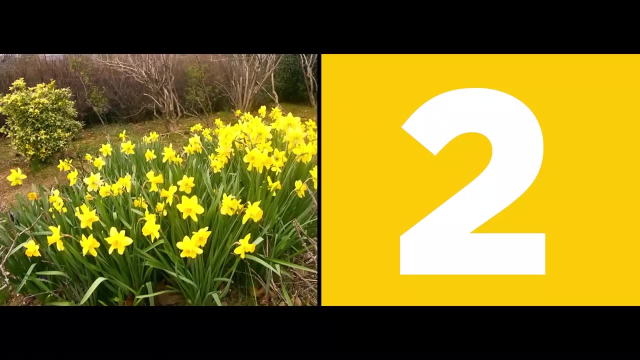 They love full sun and they can take some partial shade. If you're growing them in a shady area, they're probably not going to come back for very long. The next thing that keeps daffodils from not blooming is that over time, the clumps become well too congested. They need to be. 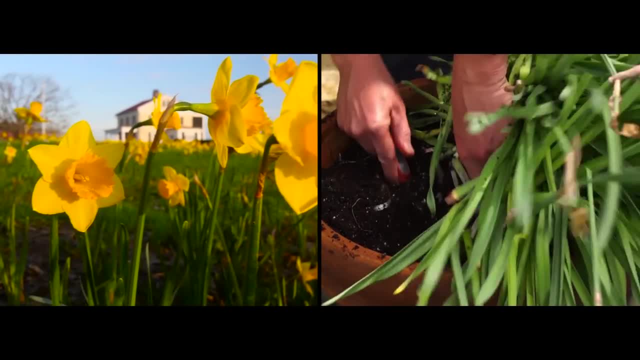 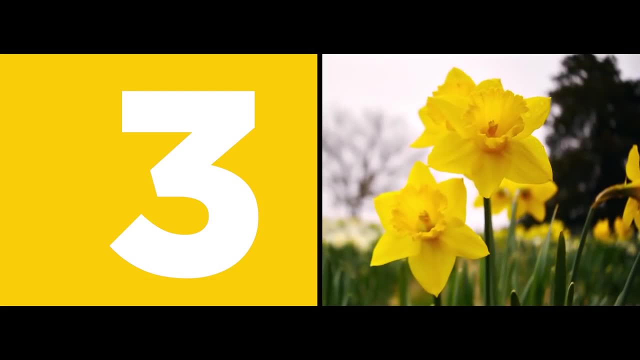 separated and divided. If you'll separate and divide them, depending on the variety, about every three to five years, you'll get clumps that are not going to come back. You'll get continuous bloom. The next or third reason daffodils don't continue to bloom is that we cut. 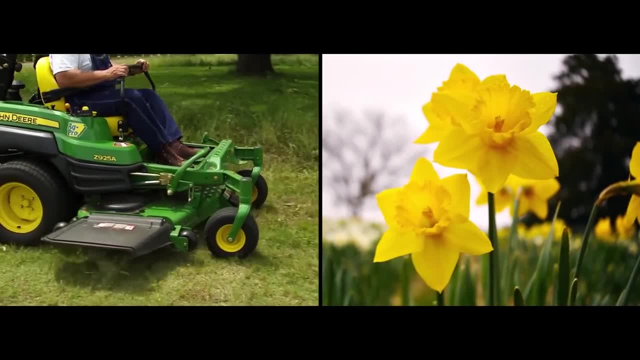 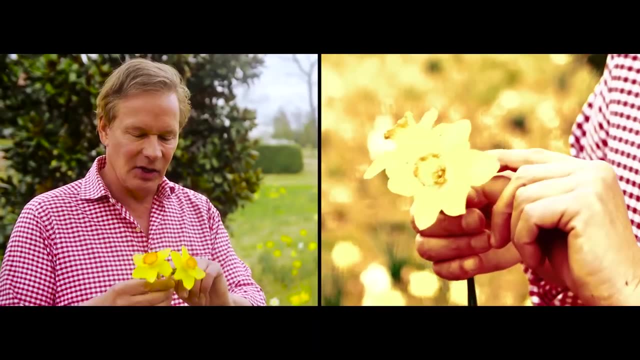 the foliage back way too soon. Let it last. In fact, let it last as long as it can. That's the best way. But if you have to cut the foliage back, let the bloom fade After that, six weeks later. you can cut the foliage back and it will not keep the flowers from blooming the next year. The fourth reason why daffodils may not bloom is they're hungry. They need to be fed. This is the time of year you can just take. 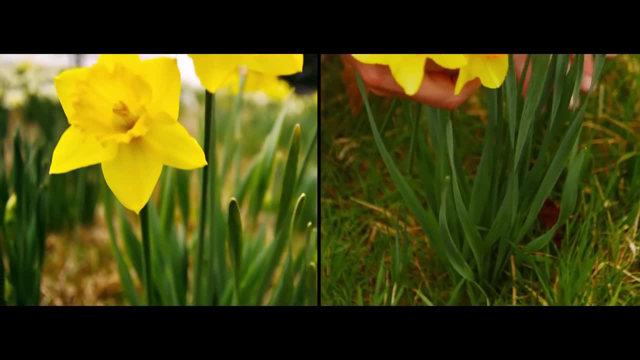 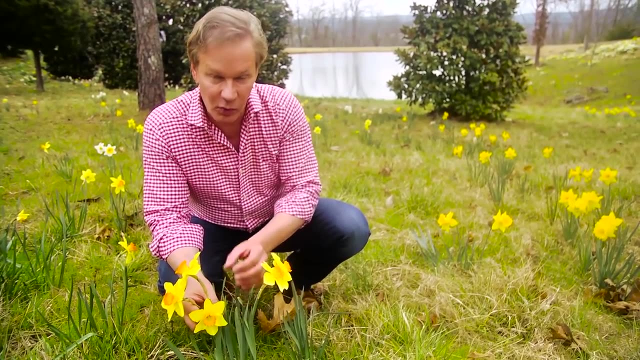 some granular fertilizer and sprinkle it around the plants, Feed the foliage and let that foliage last as long as it can. It can die back naturally. What happens is this foliage will energize those bulbs for lots of blooms next year. And the final reason: they often don't bloom. 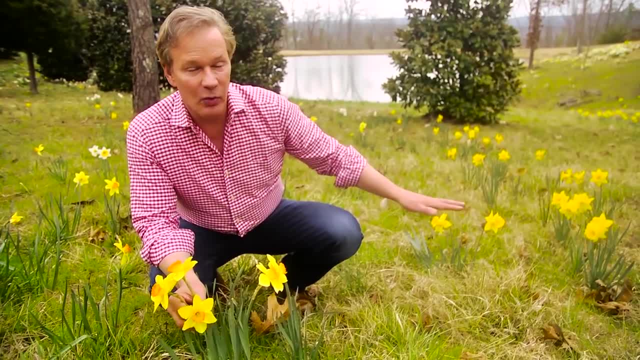 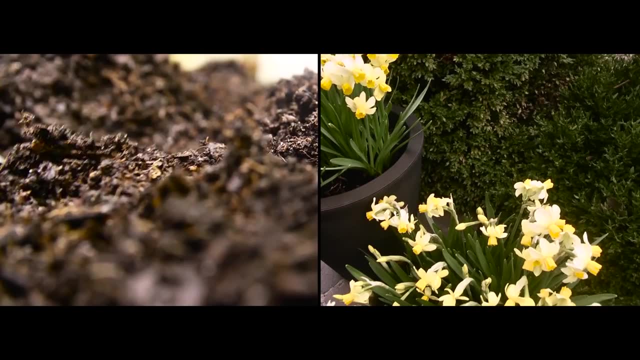 is the soil conditions aren't quite right. See how this slopes. It drains really well, But there's enough clay in the soil that it holds moisture. Daffodils do need moisture, but don't plant them where they're going to sit all winter in wet. 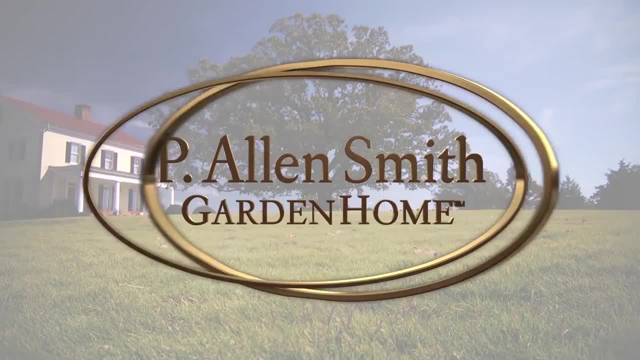 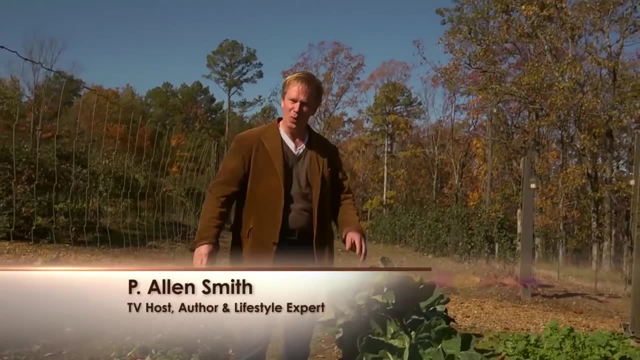 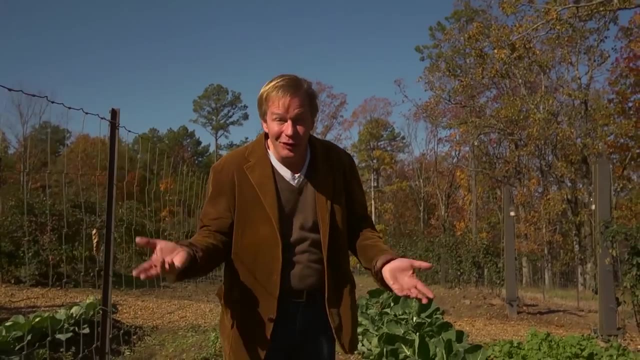 soggy soil. You know, anytime I tell someone that I plant a fall vegetable garden, they go: whoa fall. What can you grow in the fall? I thought it was getting cold. Well, there are actually vegetable plants that prefer the cool weather, I mean 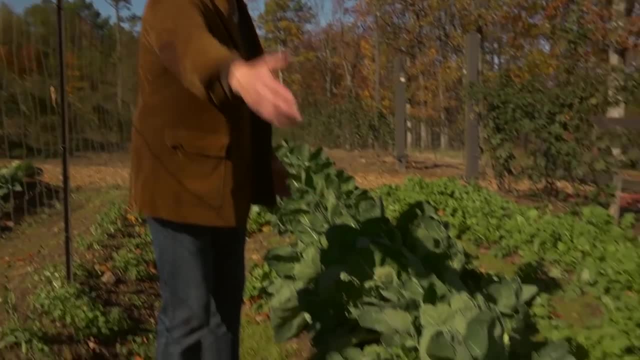 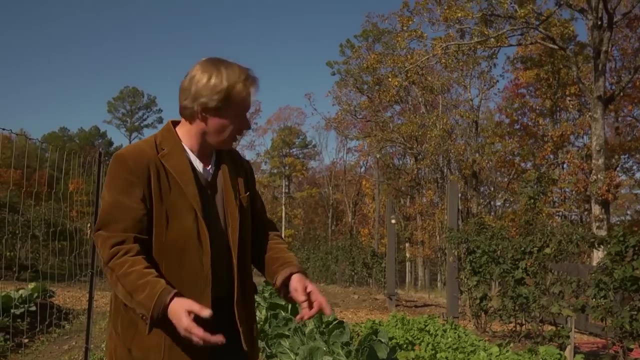 they like it cold. For instance, this Brussels sprout row I've got here. Just look at these gorgeous plants. I mean I'll grow them just to look at the beautiful plants, but they're all edible, And just over here is arugula. It likes it. cool too. So if you love rocket, that sort of. 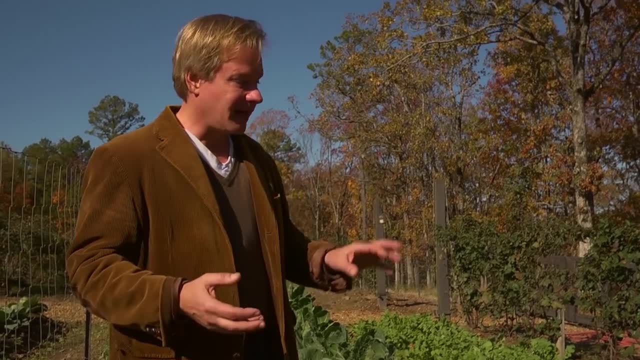 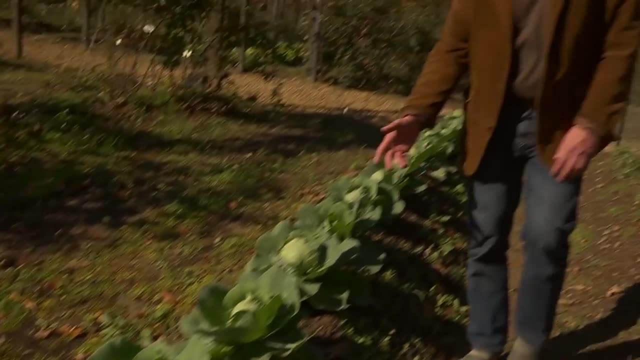 really peppery green that you can put in all kinds of salads. it's so easy to grow- I mean, it'll germinate so quickly from seeds, you can almost stand there and watch it come up. And hey, look at my cabbage. I love this little cabbage. It's called a 45-day cabbage. 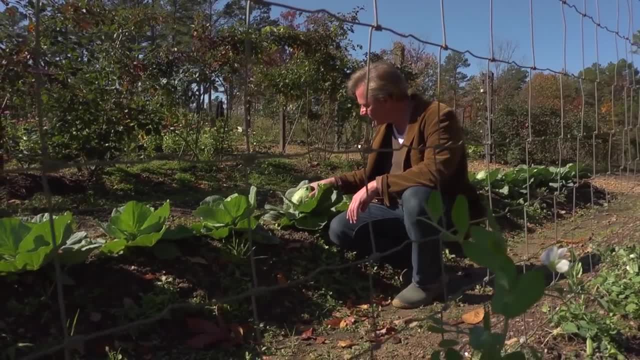 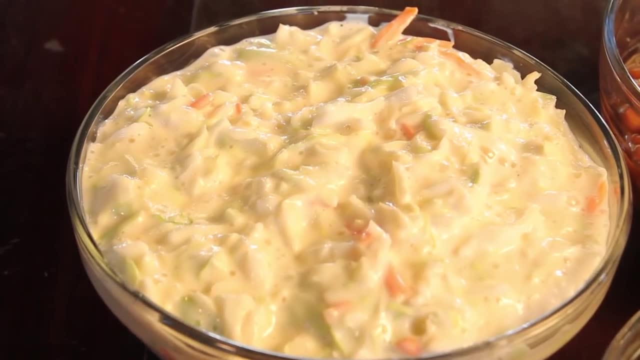 meaning that once I set out the plants, in 45 days you get a nice head And you can see firm head of cabbage forming up right here. Week or two I'll have enough cabbage here for all the swaths I can eat. I can even make sauerkraut And right next to it is ruby chard And I love the. 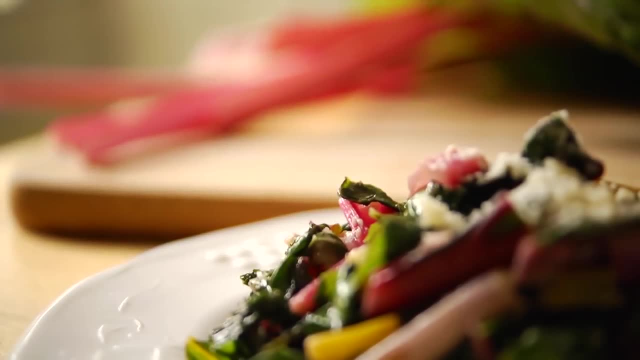 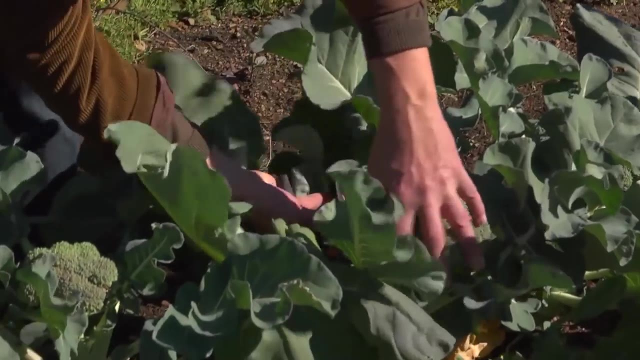 bright red stalks of the ruby chard. It's so beautiful And over here, just look how gorgeous this is And I'm telling you it is ready to pick now. Look at the head on this thing. So I'm just gonna reach in here and take that off. 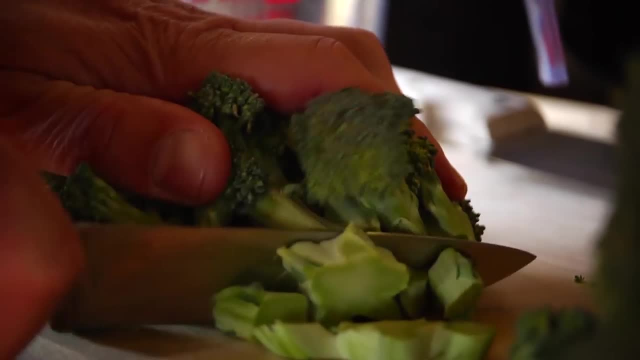 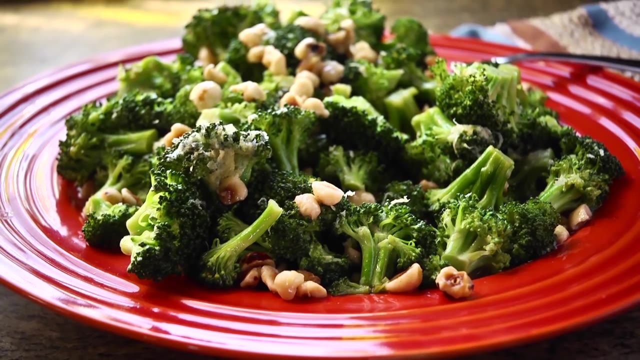 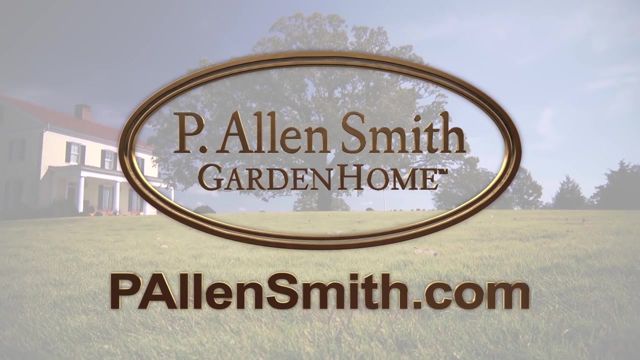 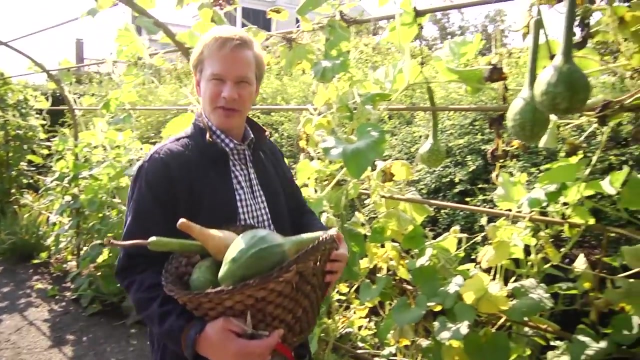 That is one beautiful head of broccoli From the garden home. I'm Allen Smith. Hey, gourd head. Why don't we take something useless and get creative? You know, gourds are pretty fascinating, I think to me because they're useless in today's society. 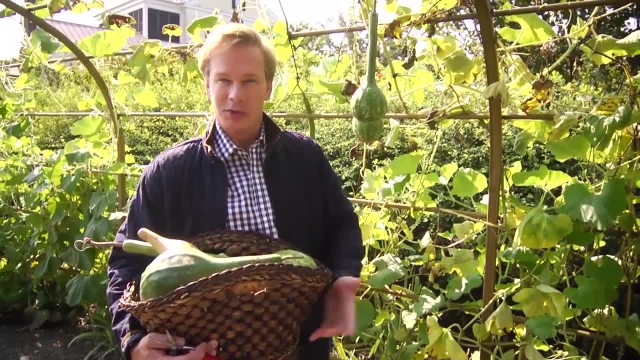 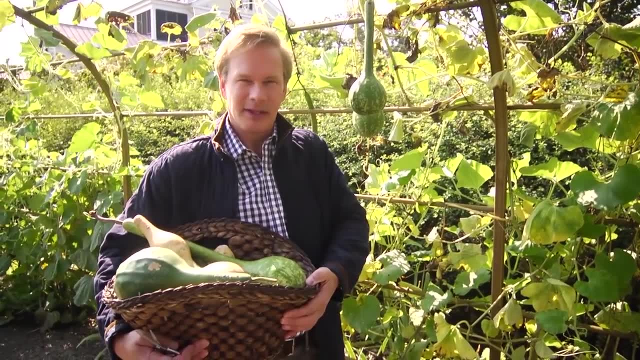 we don't need them for dippers or vessels or tools like we did thousands of years ago, But I do think they have a place when it comes to decorating. That's why I keep them around. It can be really cool. It can be really cool for any kind of table decoration you might wanna do. 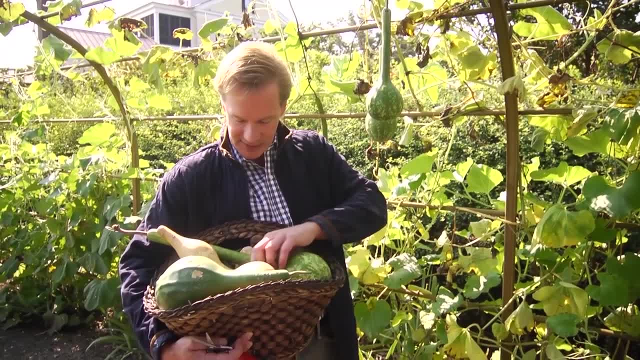 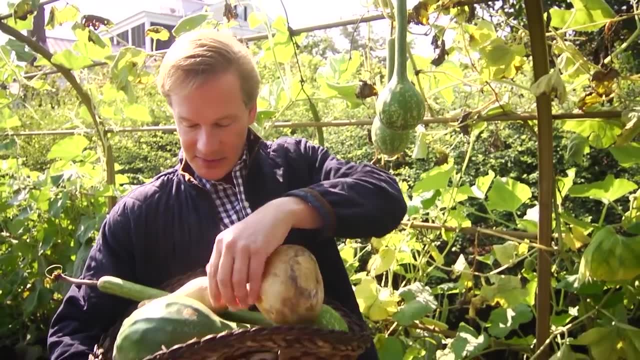 something kind of fun and funky or something for the holidays. Just look at some of these. This is a dipper gourd- It would be used to dip water. And this is a bird's nest gourd. And this is a baby caveman club gourd. We also have snake. 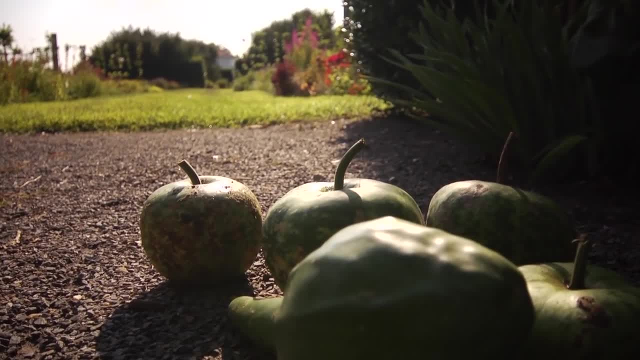 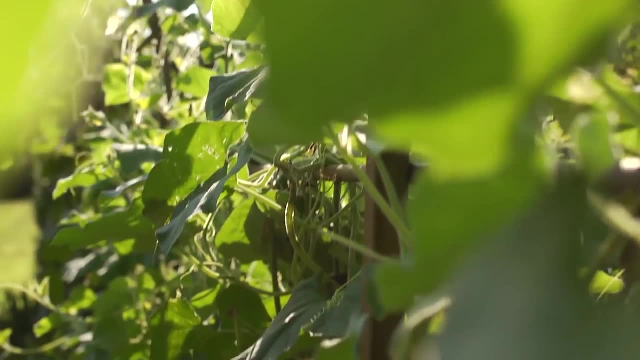 gourds, and also one called an apple gourd, growing right here on this trellis. They're wonderful. I planted them back once the soil got warm in the late spring And the vines, well, they just, They just grew like you cannot believe. And they've produced all these different gourds. 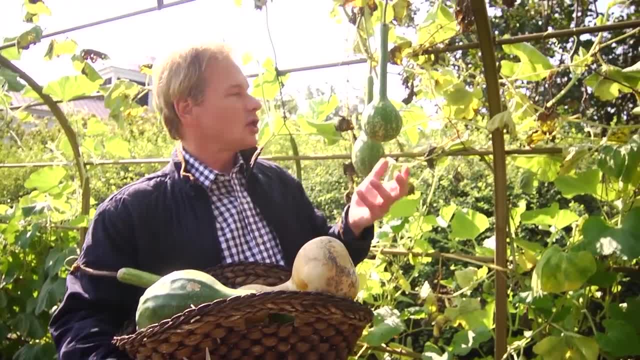 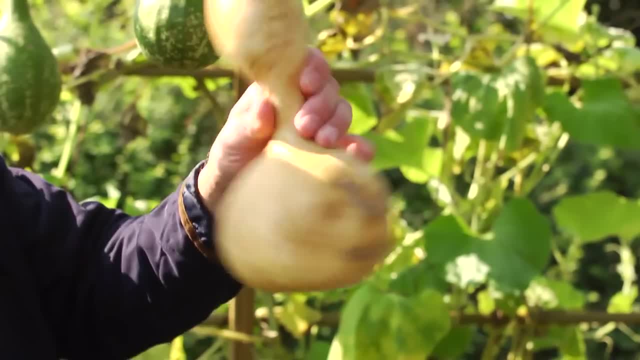 And the best time to collect them, if you wanna dry them, is when they begin to turn. Of course, I'm picking some of them green because I wanna use them for a tablescape, But what you ideally want is for them to begin to dry like this: The seed will rattle. 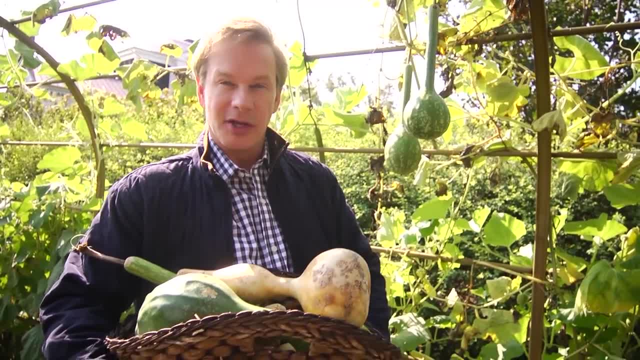 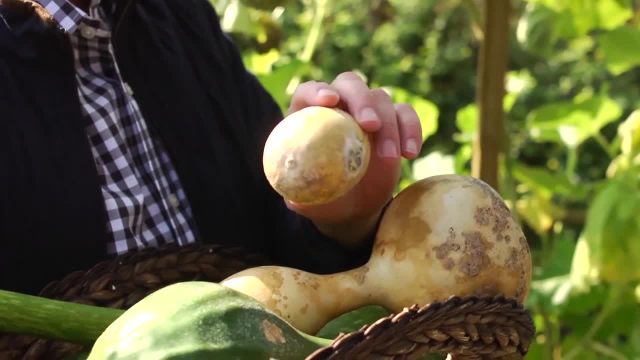 It takes about three to four months for gourds to dry. You wanna keep them in a cool, dark, dry place, And if they begin to get a little bit of mold on them, you wanna wipe them off with a dilute solution of. 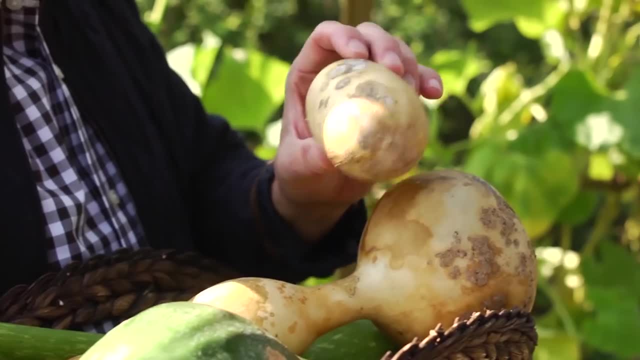 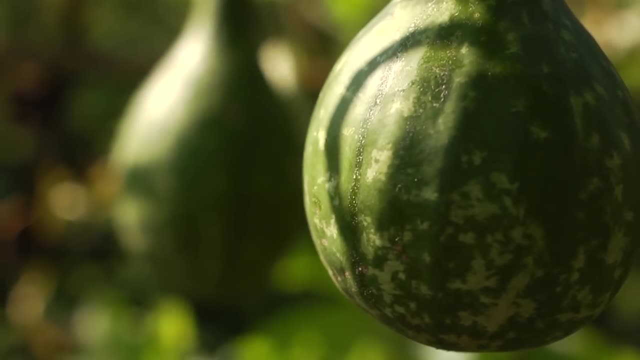 chlorine And that will keep the mold at bay and let them dry completely. Gourds are about the easiest thing you can grow. They're perfect for kids to grow. There's something magical about them. They grow like a jack in the beanstalk, really, I mean. 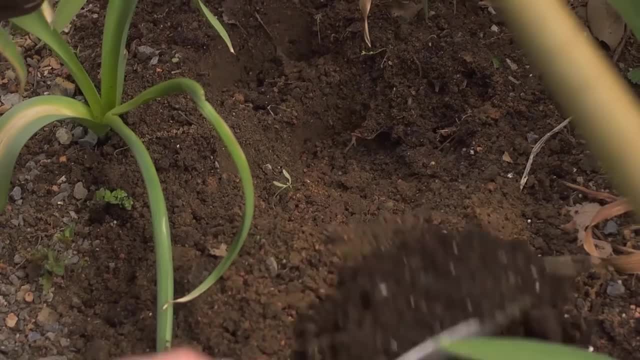 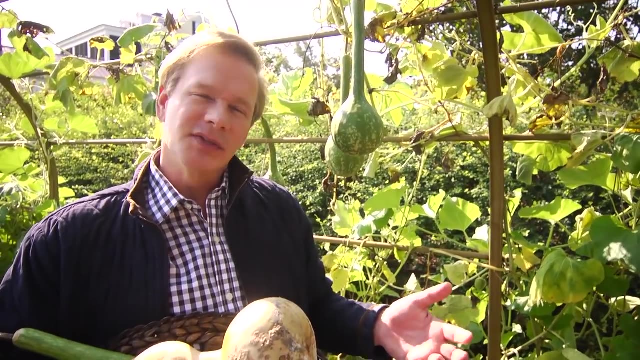 all they need is plenty of sun. You want full sun for them. The soil needs to drain, It doesn't need to hold water because the roots will rot, And you wanna make sure that the gourd's roots stay consistently moist through the growing season to get the most abundant crop. 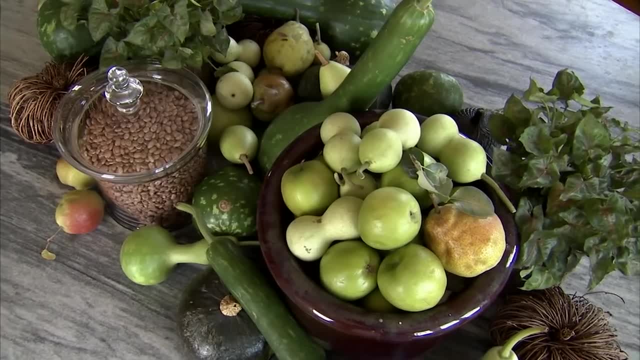 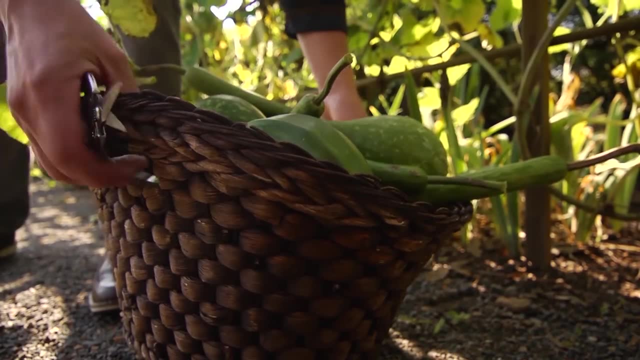 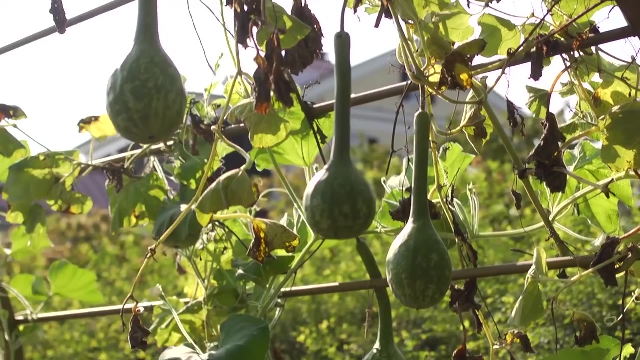 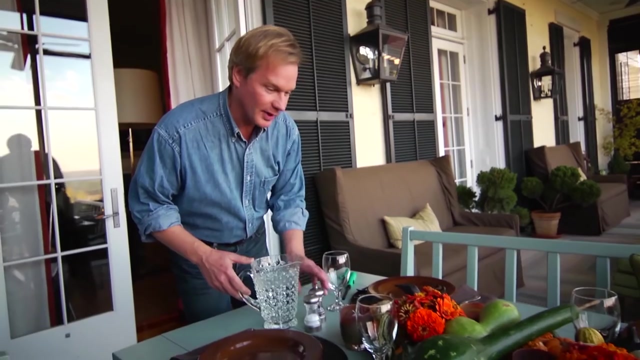 And, like I said, you can use these things for tablescapes, for table decorations, You can use them on the mantle, You can make wreaths or birdhouses. Just imagine all the possibilities with these. Well, I have some guests arriving in just a few minutes and I thought I'd go ahead and 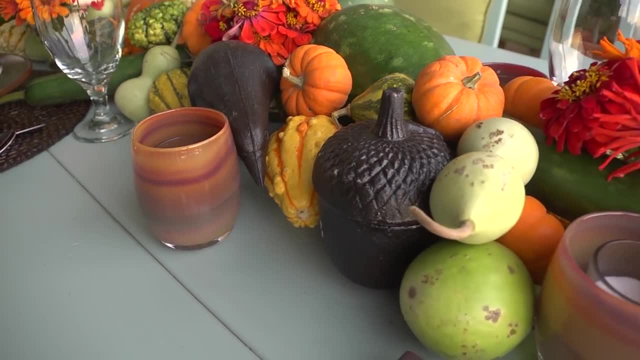 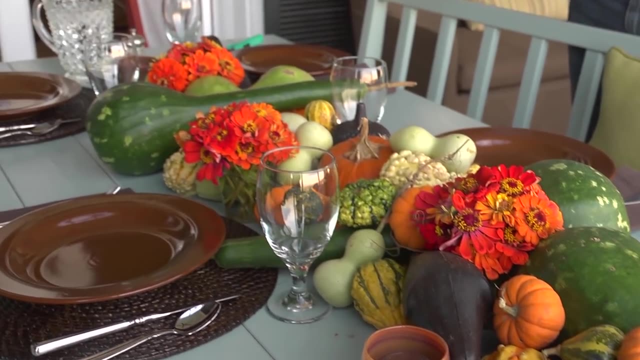 just show you how I put this table together. It's autumn and I love to entertain this time of year because there's so many wonderful colorful colors and there's such abundance that you can use. So why don't we talk about the plates first? The table's set for six. 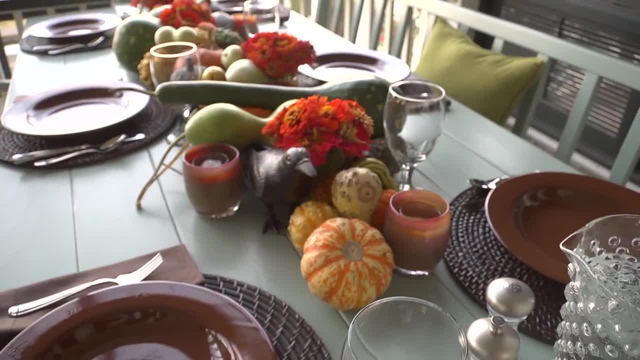 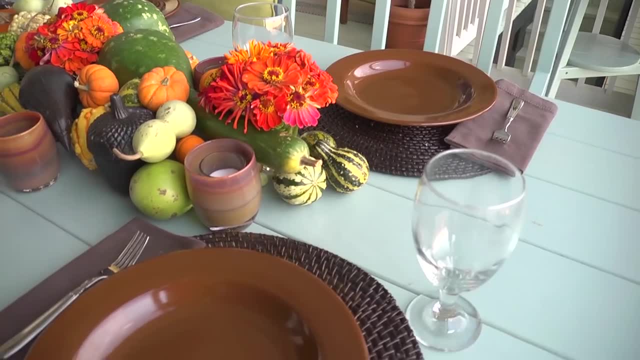 and I love to dine outside as long as I can before it gets too cold. What I have here are some round placemats that are made of a bamboo material. I love the dark, almost coffee bean brown color set against these plates, which are more of a caramel color. 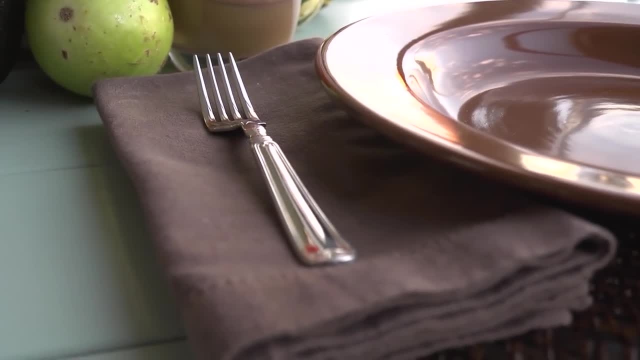 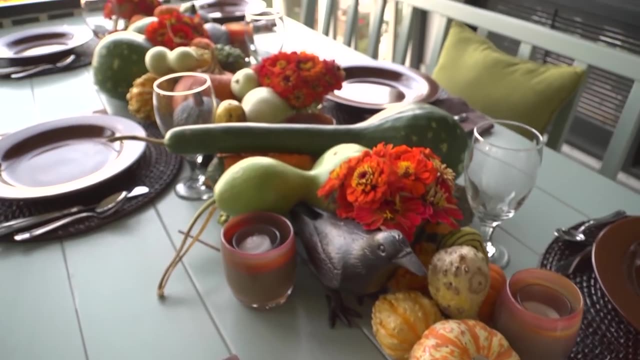 And then I've used some chocolate napkins and just some basic tableware. If you look at the center of the table, that's where it really gets interesting And this is where you can have some fun. What I did is I structured this in a way where I used large 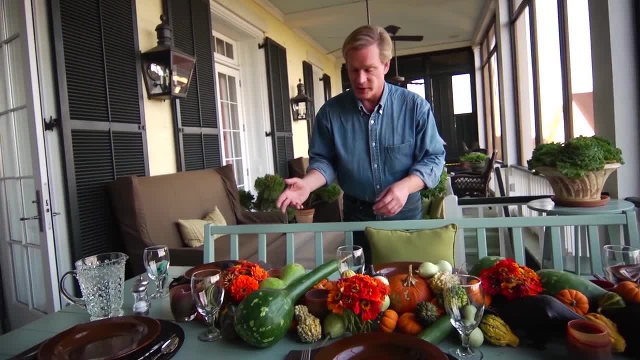 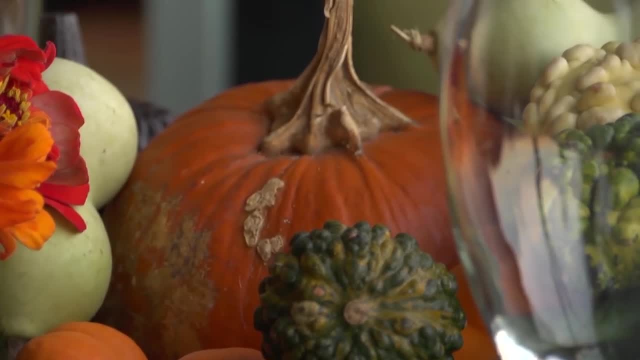 small and medium-sized objects. I started with the large objects first And you can see I used five large gourds, these big green gourds. Here's two of them here: an orange pumpkin, and then two more green gourds, as you can see here, And then the next size object would be. 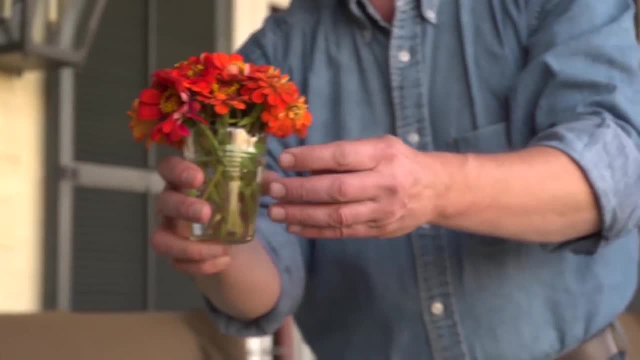 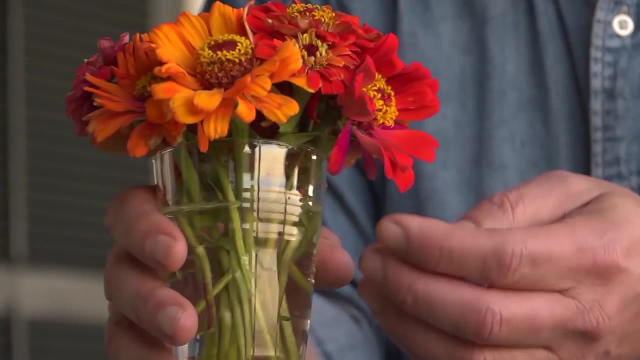 these bouquets. I love zinnias. Of course, it seems like the chrysanthemum is the flower for the fall season, but I love zinnias And they're so easy to grow. You see, the seed will germinate in 5 to 10 days. 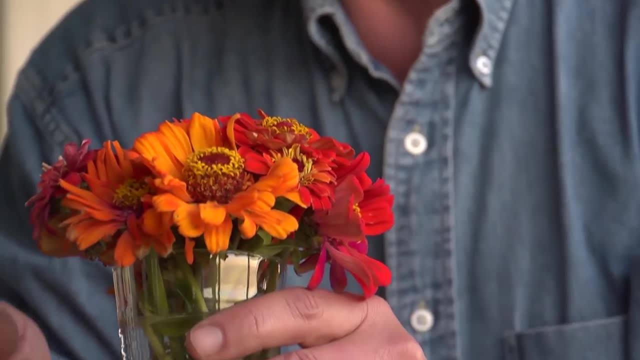 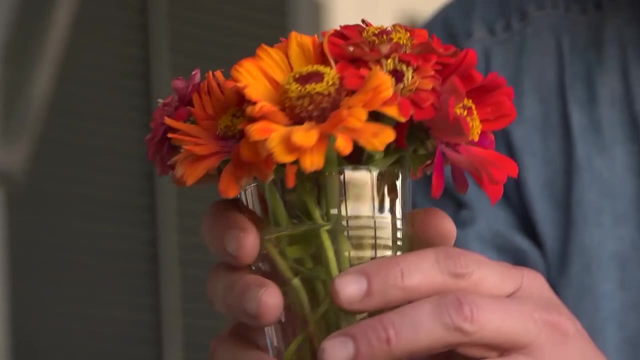 and you can have flowers in as few as 35 days, up to 60 days, And I like to plant these in late summer, particularly these autumnal colors. They're really beautiful And you can take about 25 blooms and gather them together in the garden and bundle them And just place them in. 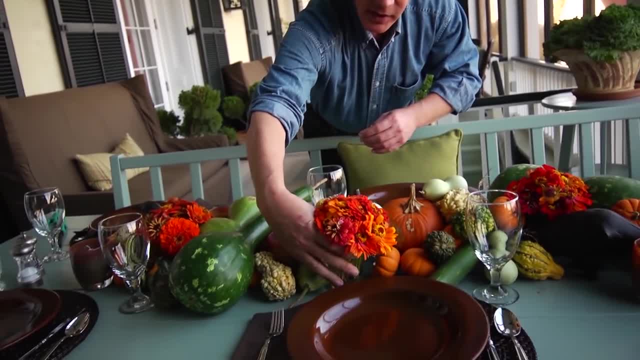 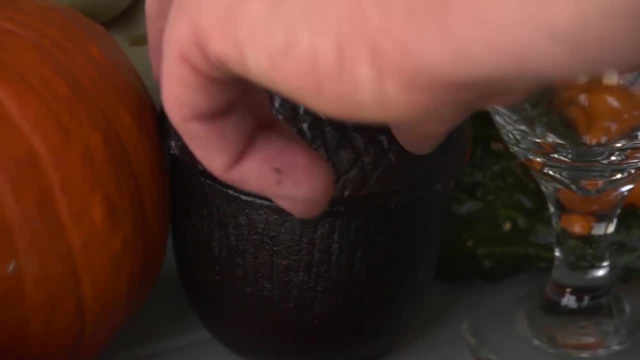 a clear glass, as I've done here, and just tuck them in among those large gourds. Then I equally distributed some of these cast iron pieces, crow and this acorn, And you see, I used four of those because I have a pair of each Crow here. 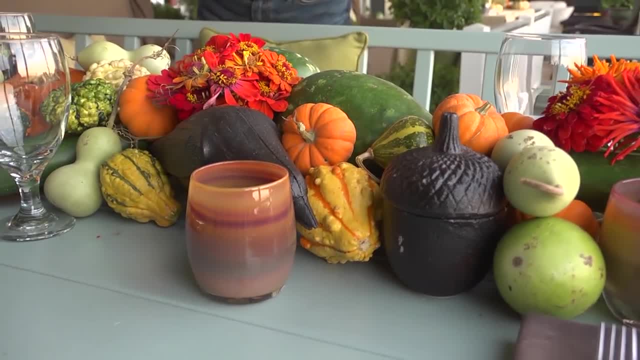 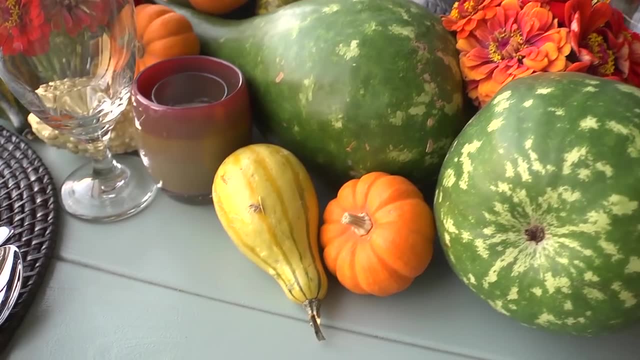 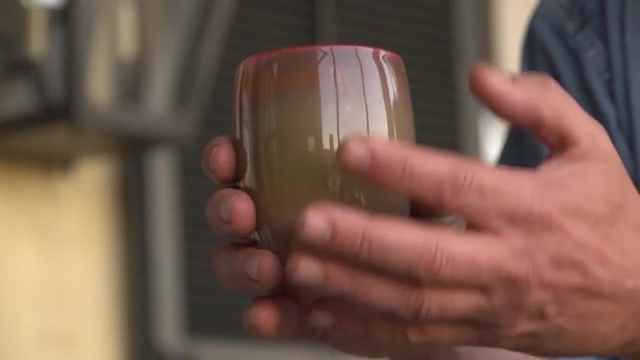 acorn crow and acorn there. So I created the structure And then I filled in with 45 of these little gourds and just tucked them in all these different, various places. And right on the outer edge I used these glass candle holders, which I love Because as they warm these earth tones, 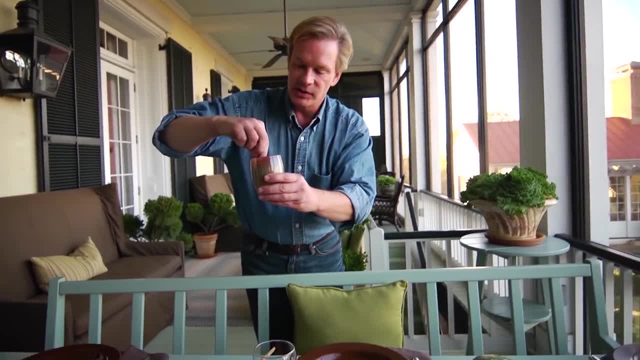 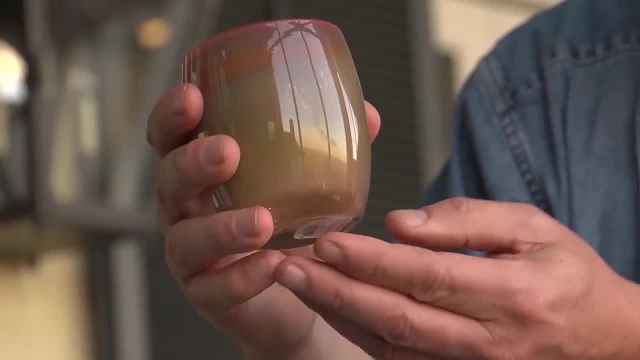 begin to illuminate the entire table. What I like to do is take a clear glass of otive and drop it inside here, because I don't want the fire to shatter these gorgeous containers. As you can see, I kept the entire arrangement very low. I assembled the large 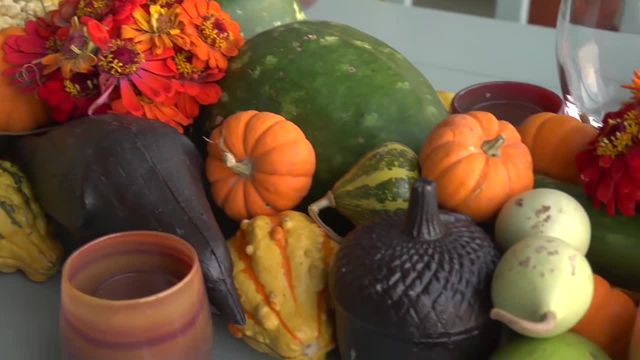 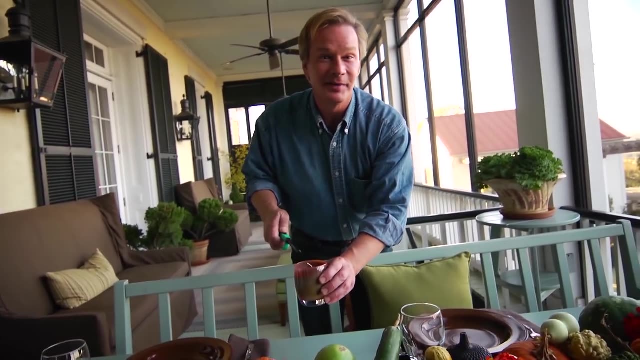 things first brought in the medium-sized objects and then repeated them all the way down, And then the last touch is to illuminate them with these candles. I better get these lighted, because I've got guests coming in just a few minutes. You know, you can use apples for a lot more than just eating. 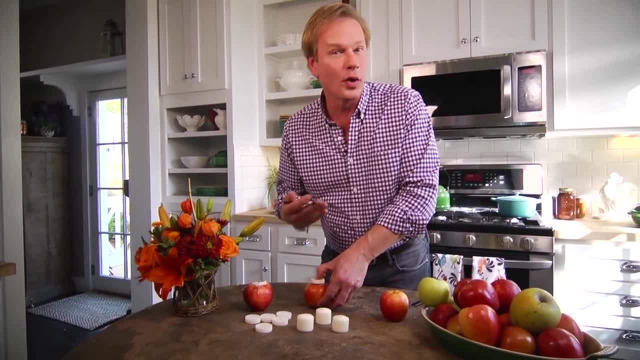 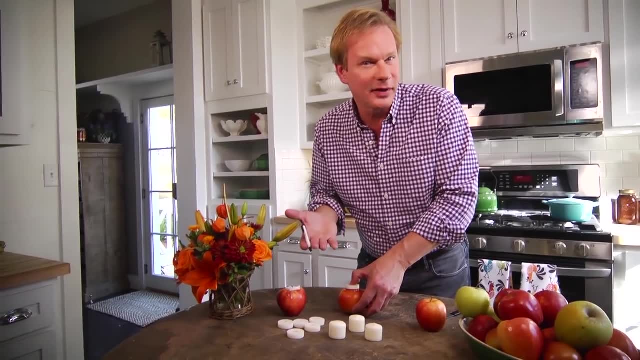 You know I'm always looking for interesting ways to display ordinary things like candles on a table for a party. So it's the fall of the year. what's plentiful out there? Certainly apples. You can find them in a farmers market, a farm stand. You can go to the orchard or you can just pick. 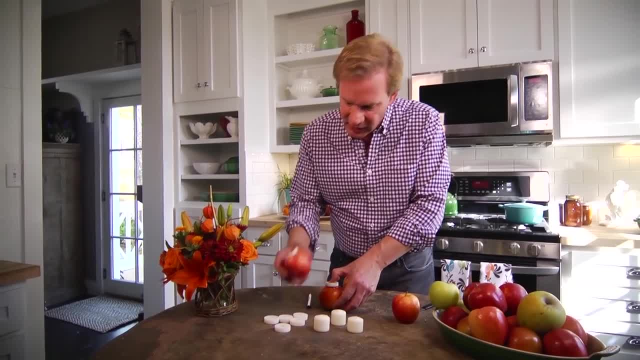 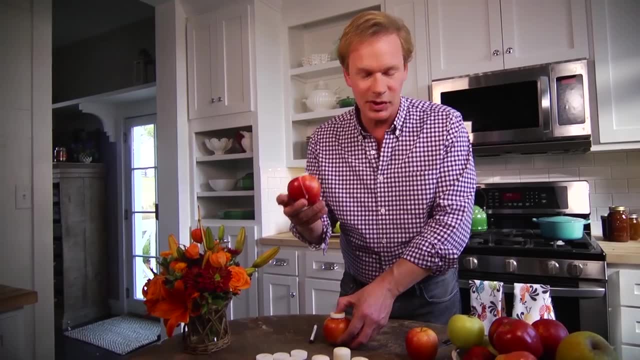 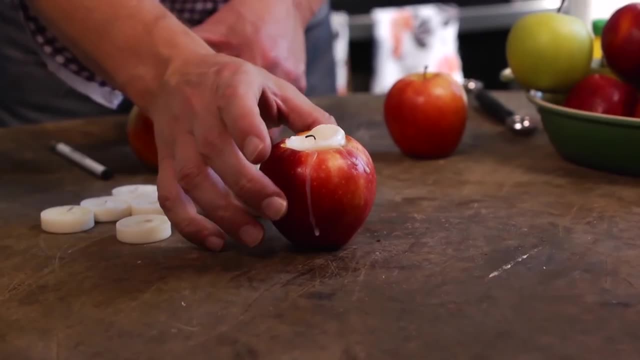 them up in the grocery store. What I'm doing here is I'm actually making some little apple candle holders for a festive table decoration. These are really easy to make, And let me just show you. Well, you want to make sure that apple will sit by itself and sit upright, so it doesn't. 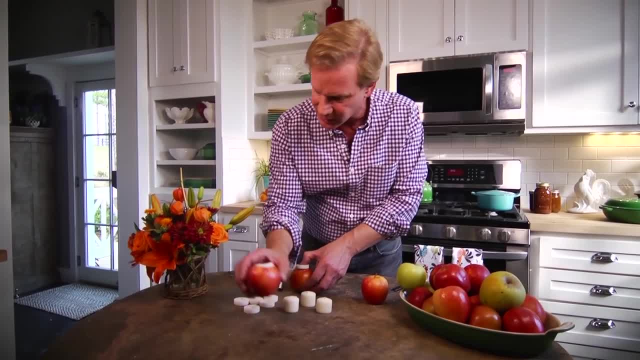 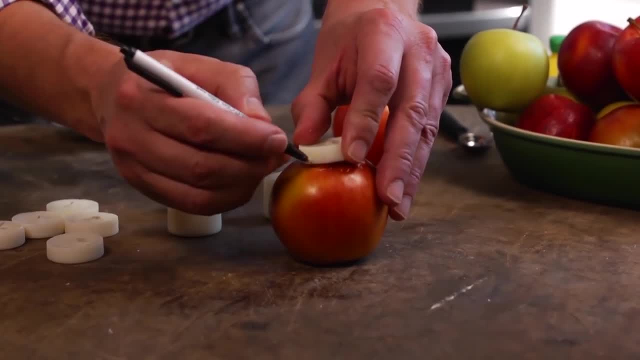 roll around on the table. for obvious reasons, This one is doing a sterling job And I have one here that I've just placed a votive candle on the top And I used a pen just to go around and score the exact diameter of it. 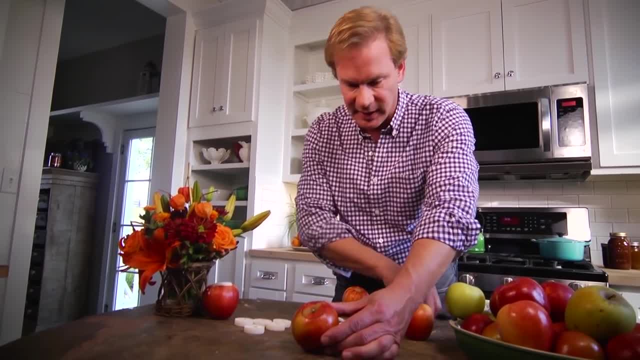 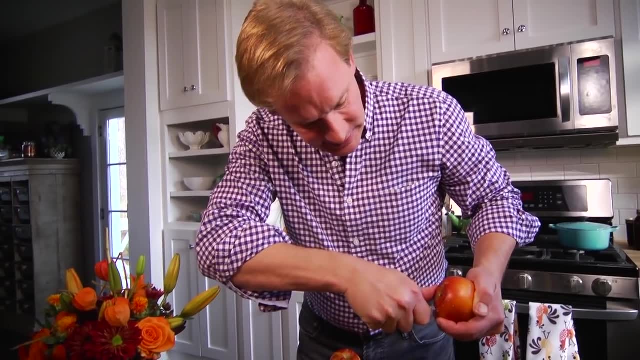 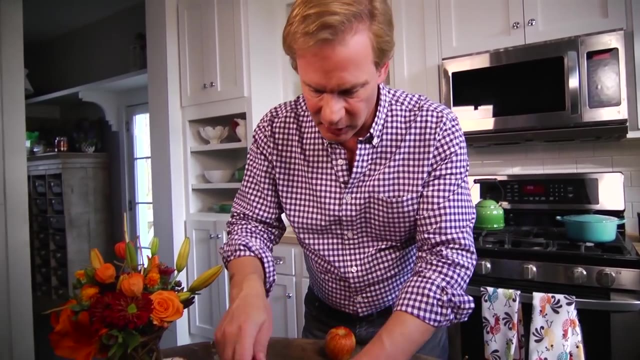 And you can see that circle there. Now it's just a matter of taking a little paring knife and cutting directly into the apple, straight in, like this, and cutting very carefully around the edge, And then you can take a melon baller which has a sharp edge and you can just take out. 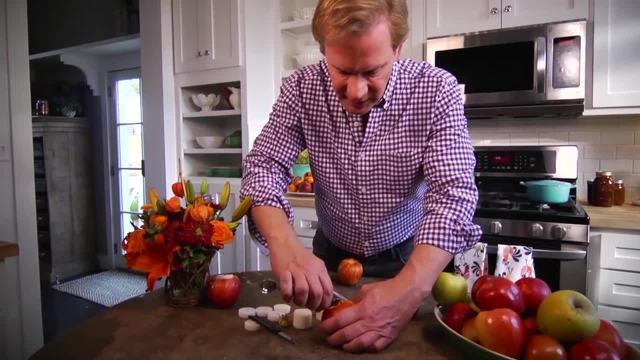 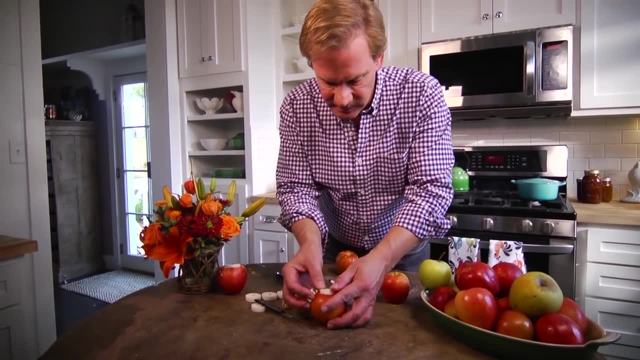 that core of the apple. See how simple this is. You get a nice clean cut edge with this melon baller. Okay, then it's just a matter of sort of sizing the candle. It's better not to make it too large in the beginning, because you could always cut it. 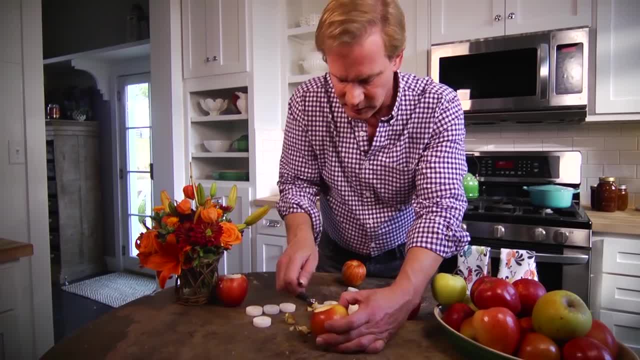 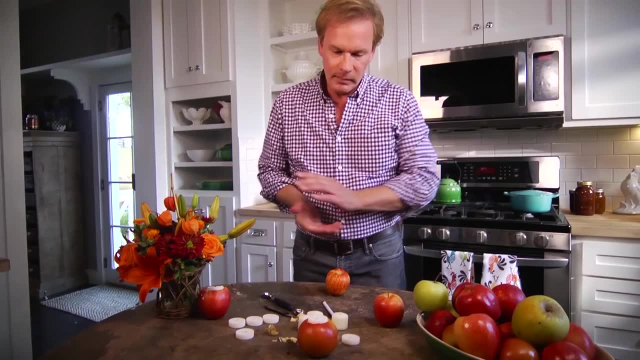 out, But you can't put it back in there. Alright, so there we go. You can see that fits just about right with just a little pressure, What I like to do to keep the edges of the apple from shriveling because we've cut into. 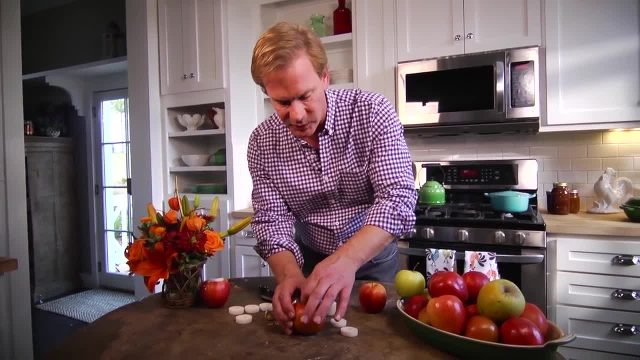 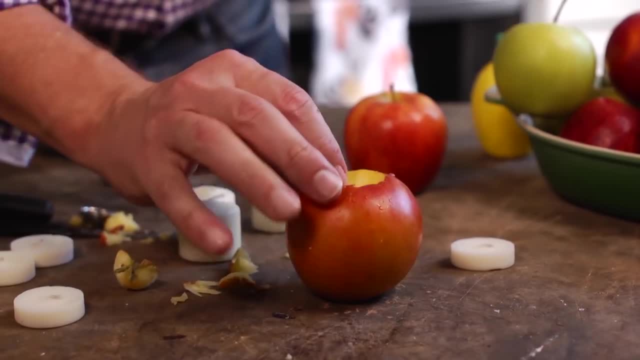 it. it's likely to dehydrate and it will discolor, as we know apples will. You can take just a little bit of lemon juice like this and apply it to the flesh of the apple like that. That'll keep it from discoloring, at least for your party. 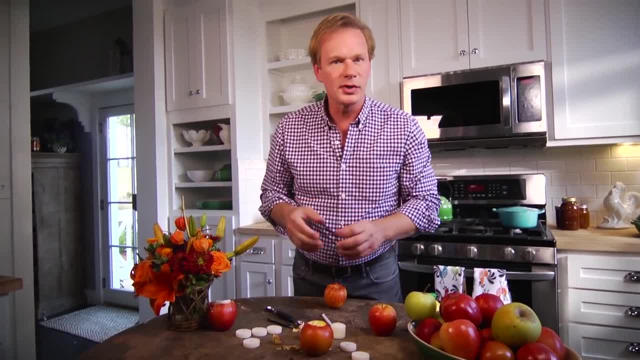 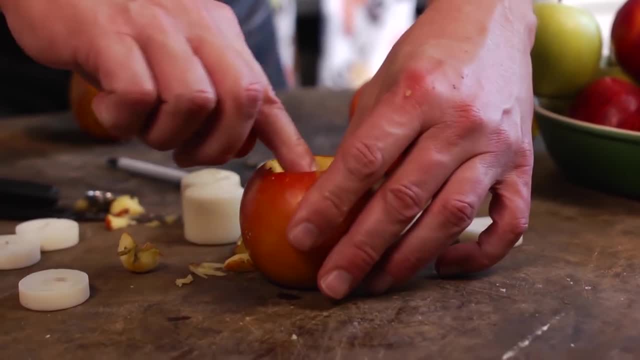 Now the other thing that I've done with pumpkins and acorn squash and things like that that I've cut. you can actually take a little petroleum jelly or Vaseline and rub right around the edge and that will seal this off and keep it from losing moisture and shriveling around. 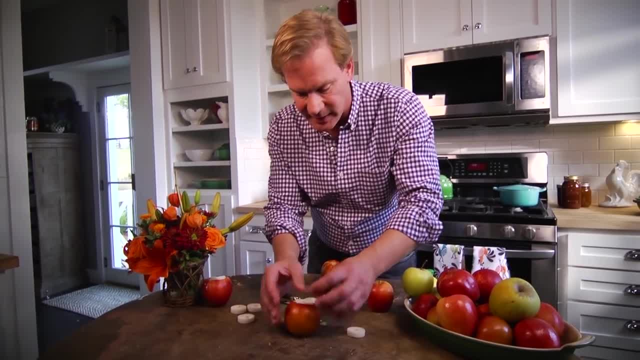 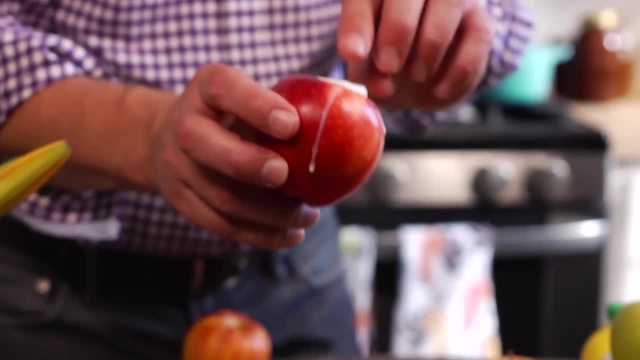 the edge. Just another little tip. You see, this sits in just like that and then you can light it. You can let some of the candle wax drip around the edges, like I have here, to sort of seal that gap, If there is one, between the candle and the apple itself. 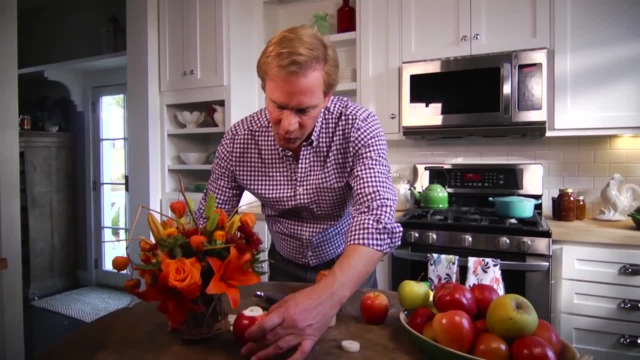 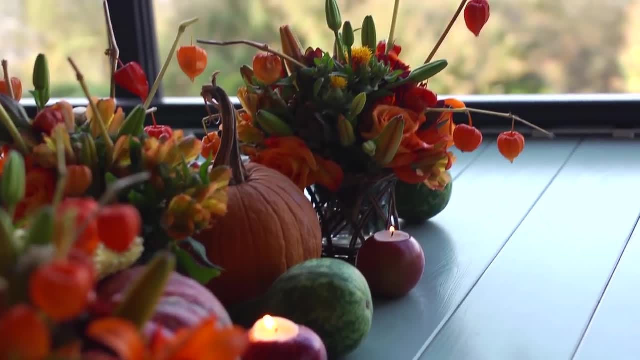 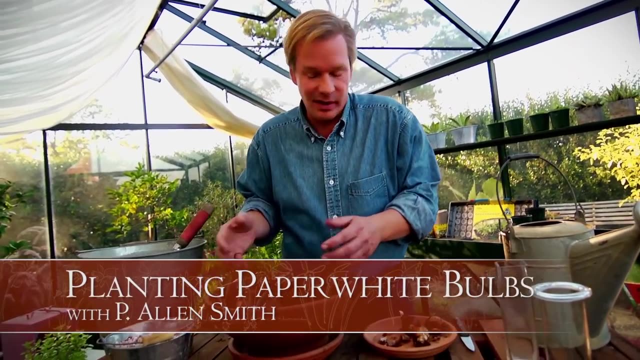 Now you can see I have an arrangement here that the colors work beautifully with this. Just imagine these lining a table all lighted with these beautiful arrangements. It can make a magical table setting. There are all kinds of winter projects you can do to bring life or a little bit of the. 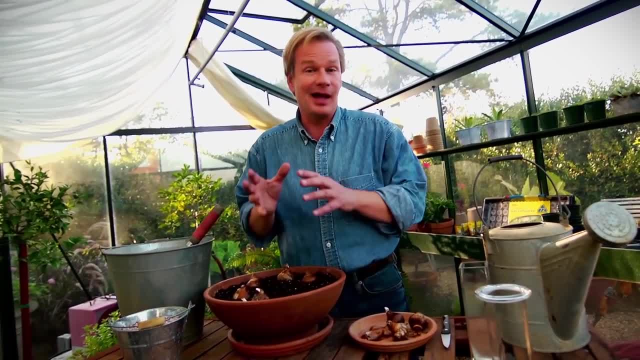 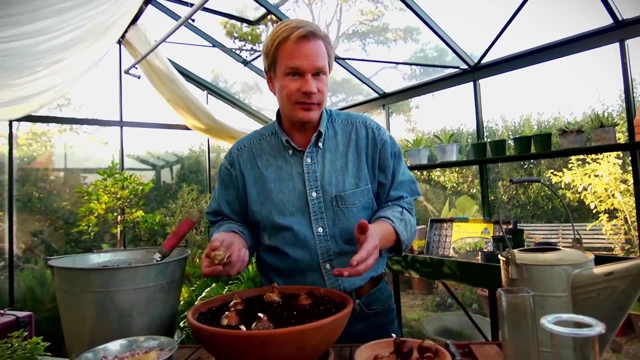 garden into the home. One of the simplest is to just take a flower bulb, like one of these paper white narcissus, and light it up, Then grow them into something gorgeous and fragrant. Now, what's interesting about paper whites is that you can grow them as long as you give. 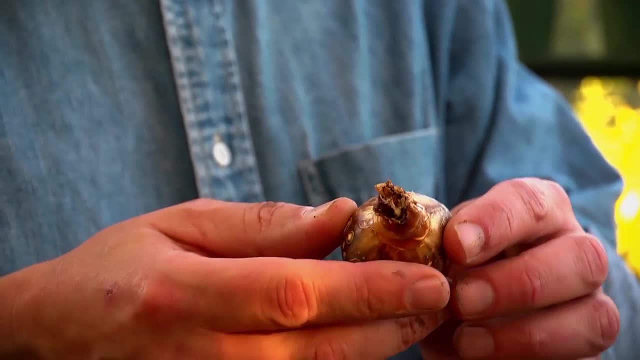 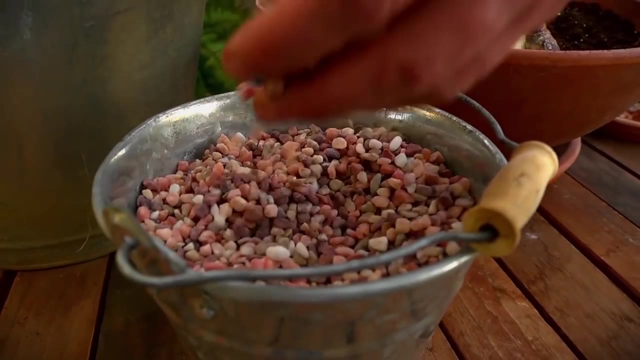 them a little water and a little light and some warmth. What I'm talking about here is, once you apply water to whatever medium you're growing them in, whether it's soil like this or gravel, or just water alone, they will begin to germinate. 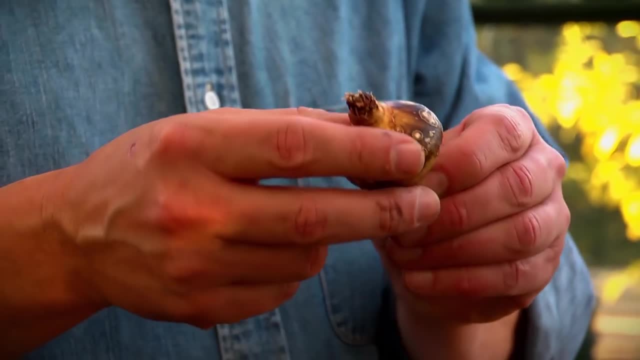 and bloom within six weeks. Okay, And you want to make sure that the temperature for the paper whites is between six and a half degrees, The temperature for the paper whites is between 65 and 75 degrees and you don't want to keep. 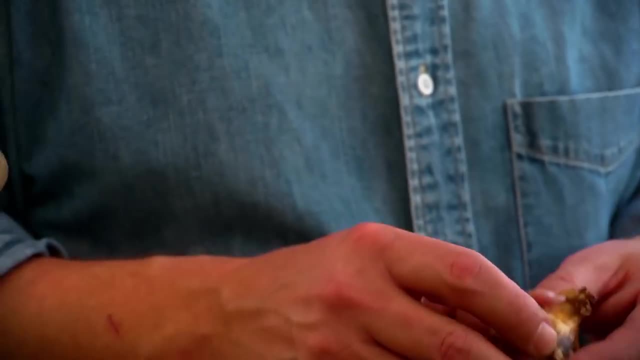 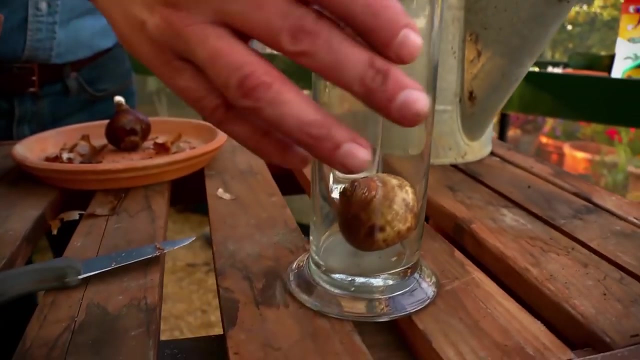 them in direct sunlight. Now I grow these in lots of different ways. I like to mass them in a big bowl, like you see here, growing in soil, Or you can take a bulb and drop it in a glass container like that, add a little water. 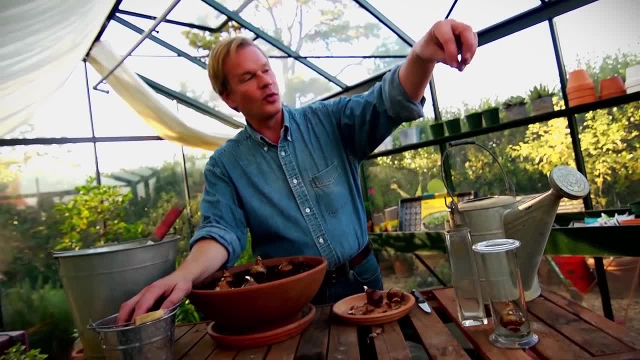 You can even pour some gravel over the top and that flower will grow right out of the top and bloom. They're really indestructible. You see, what's great about them is that the flower is already in the bottom of the container. 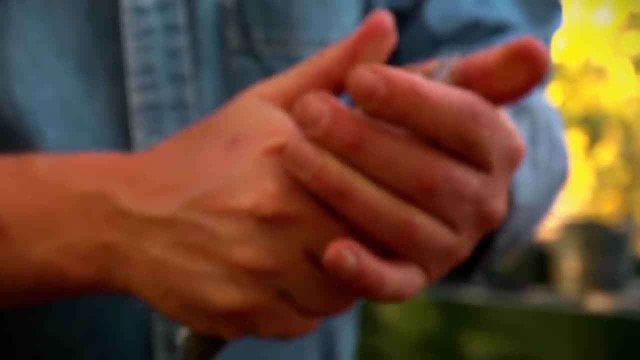 You don't have to worry about that. You can just take a little bit of water and you can just pour some gravel over the top and that flower will grow right out of the top and bloom. They're really indestructible, So you can just put them in the bulb. 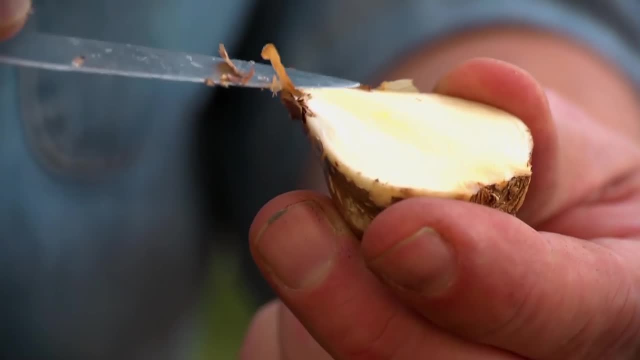 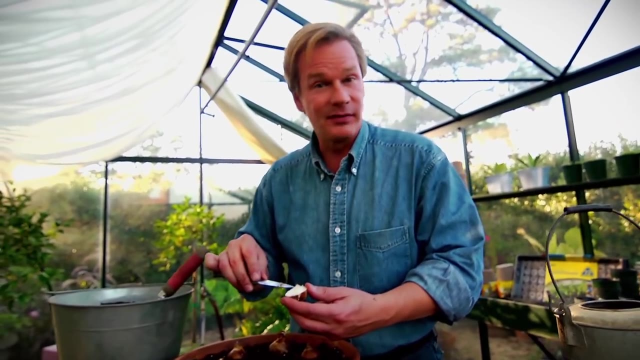 And I'm going to sacrifice this one just to show you the baby flower. You see, right there There's the embryo of that flower And all you have to do is give it some moisture, give it the temperature I just described and some sunlight, and it will begin to grow and flower for you. 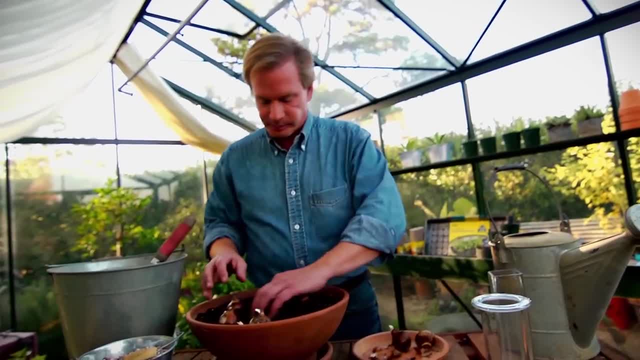 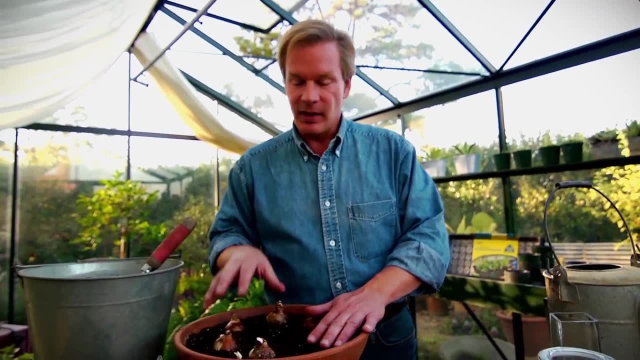 Now one thing that you can do is you can take these and plant them in containers and stage them. If you keep them slightly cooler, you're going to slow down the growth. What I like to do is plant, On a weekend, two or three containers and then stagger them as I bring them into the 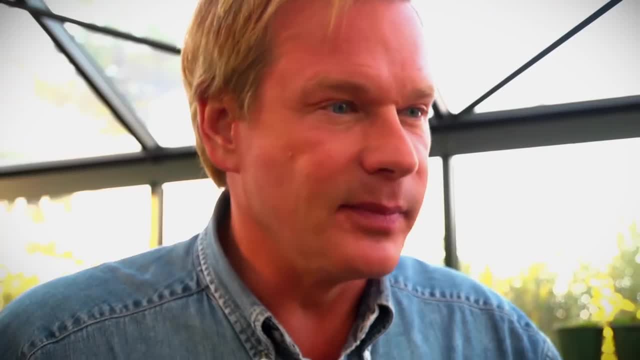 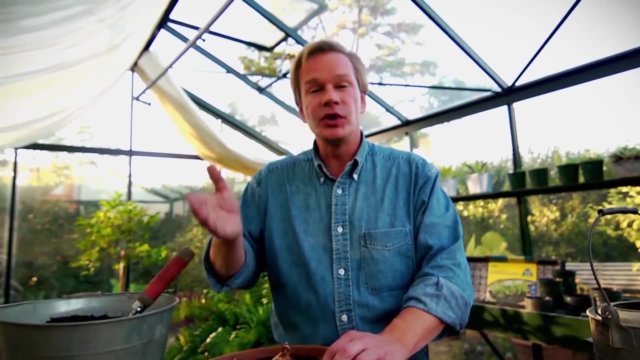 house, So I can keep them in sort of a cool area like the garage and then bring them into the house where the temperature is in that 65 to 75 degree range and they'll bloom. So you can have sequential blooms all the way through the winter. So make sure you buy plenty of bulbs and keep them in storage in the refrigerator. Now one last point: If you store them in the refrigerator, you want to make sure that they're not in contact with- They're really in the same refrigerator with apples or produce that give off ethylene gas. 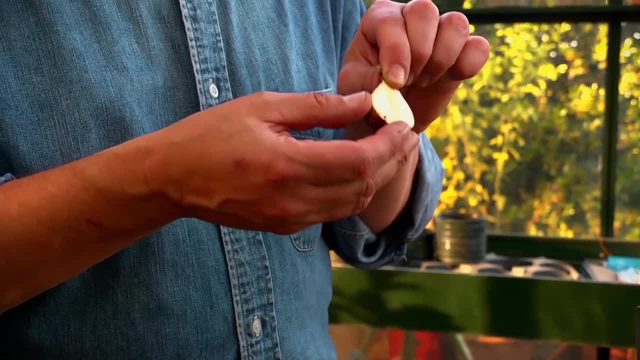 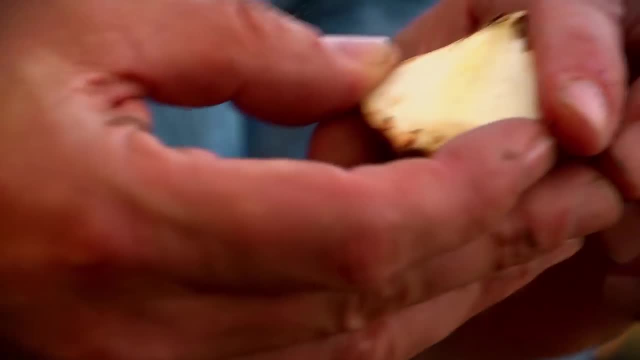 because that little embryo that I showed you will be destroyed by that gas. So if you can keep your paper white bulbs- or any other bulb for that matter- in a refrigerator where they're alone and they're isolated, they're going to do much better for you. 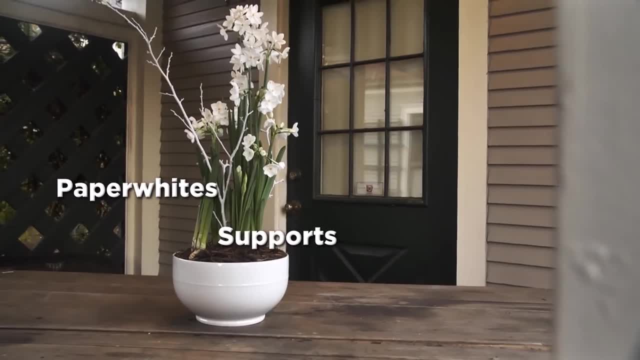 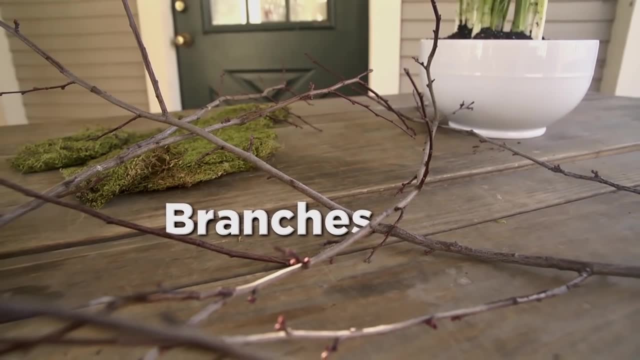 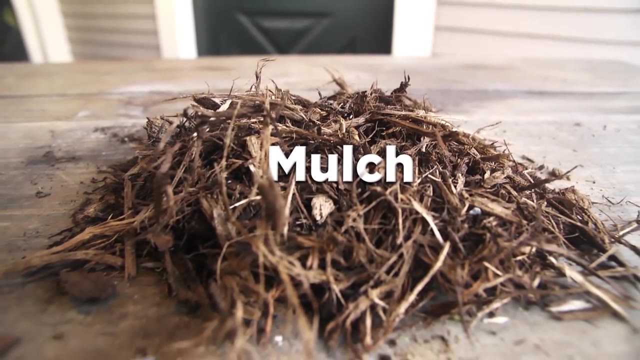 Under the same circumstances, the ingredients are going to be completely dry, and so the amount of air in the room is going to be too much for you. so you're going to have to wait a few days, And if you want to keep it like that, then keep it in a-. 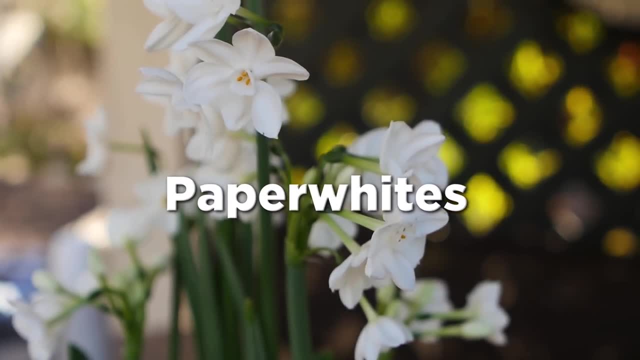 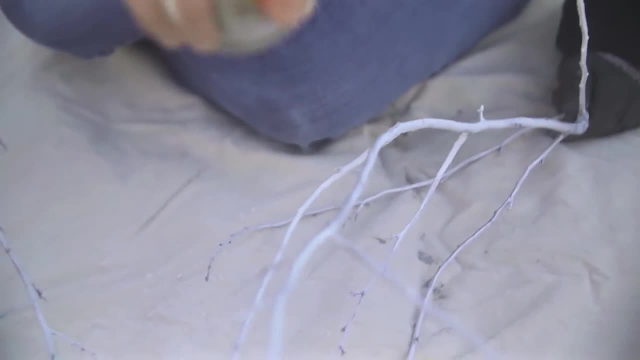 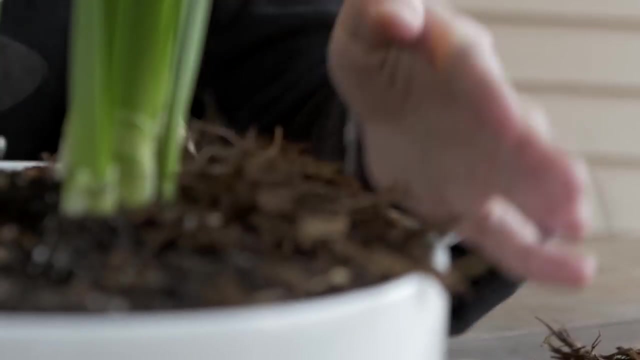 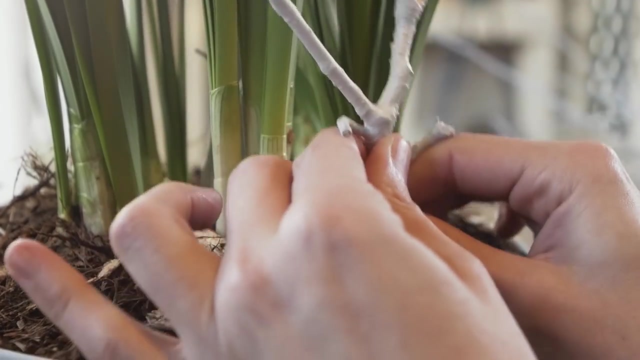 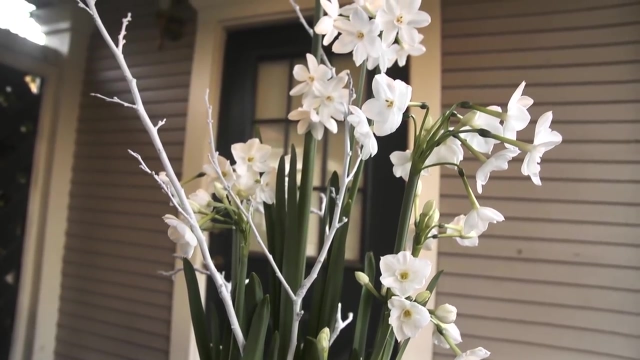 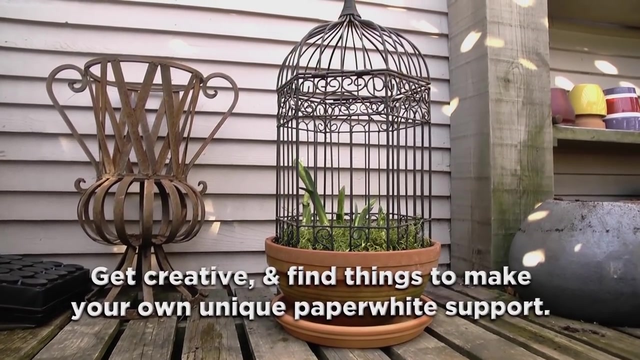 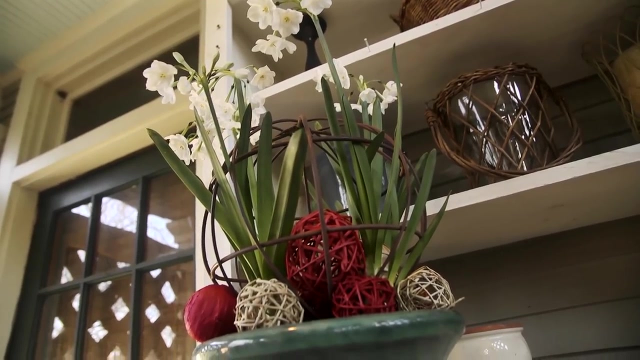 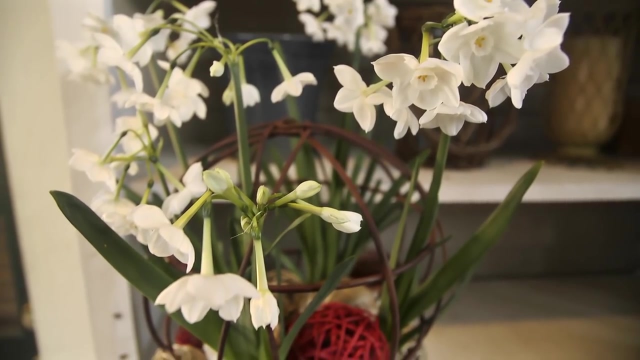 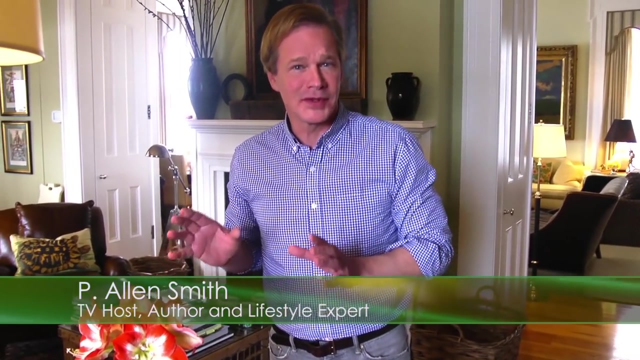 If you want to keep it a year, then you're going to have to wait a few days, Okay. If you want to keep it a year, then you have to wait a few days, Okay, Thank you. I have to tell you the amaryllis is one of the most rewarding plants that I grow in my 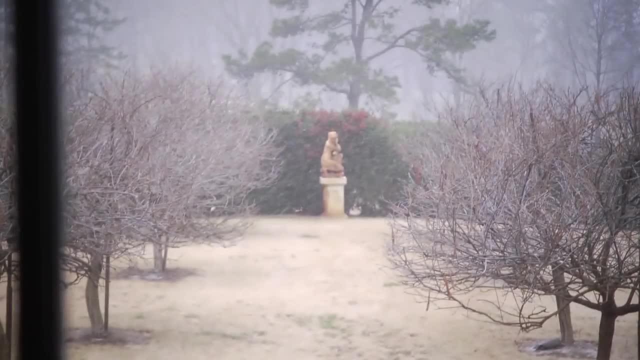 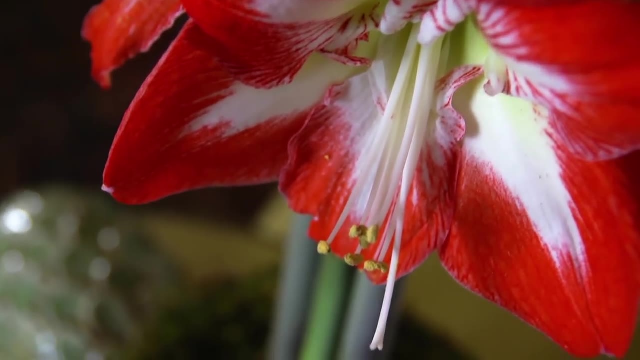 house during the winter when it's really bleak outside. Just look at the flower power here. This bi-colored variety is called Minerva. There's so many different colors of amaryllis to choose from. You know what's fascinating about it is, while I've got these planted in some soil, you actually 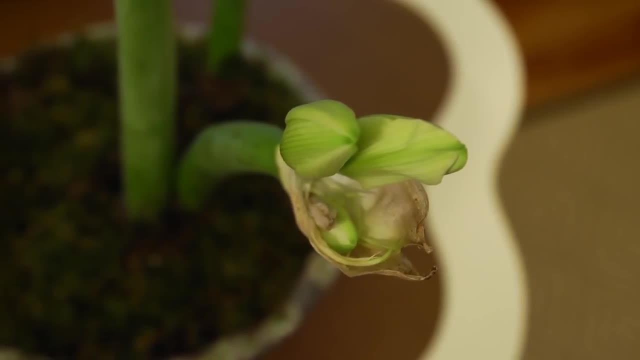 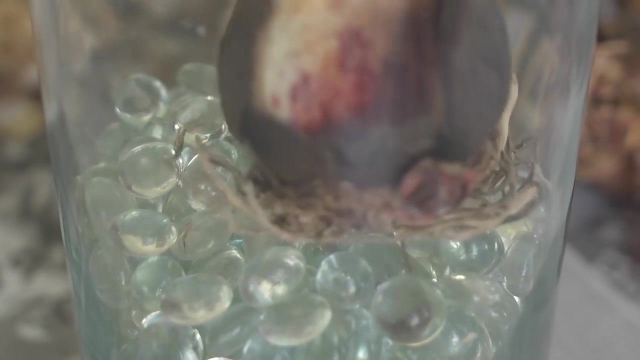 don't have to have soil to grow them and get them to bloom. If you take this soilless approach, just be sure to place beads, rocks or other materials in the bottom of your container to keep the bulb from actually sitting in water. 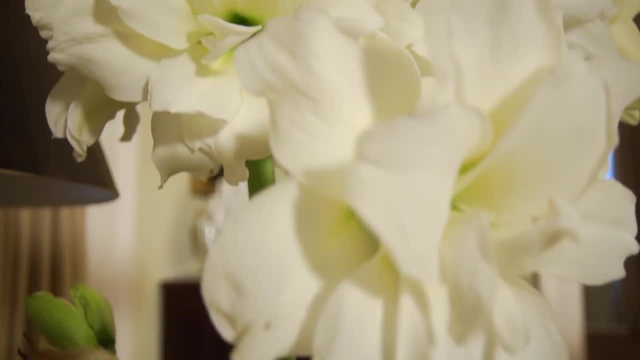 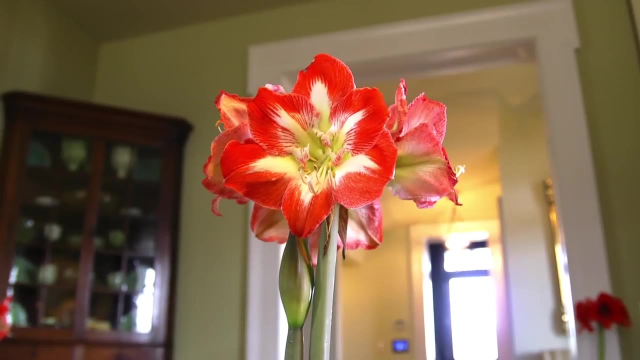 Now, to keep these flowers looking their best, place them in a cooler location in your home that doesn't get a lot of direct sunlight. Now here's a little tip I want you to keep in mind. All plants are phototropic, meaning they lean toward the light, and amaryllis certainly. 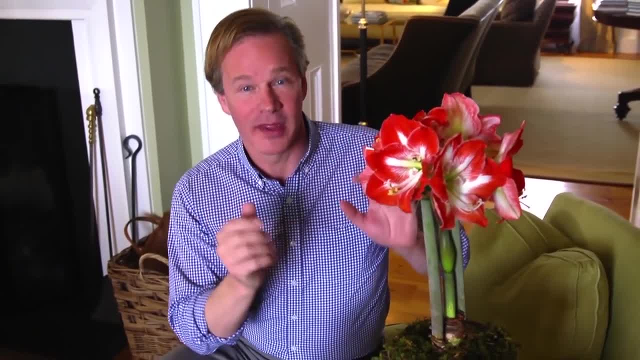 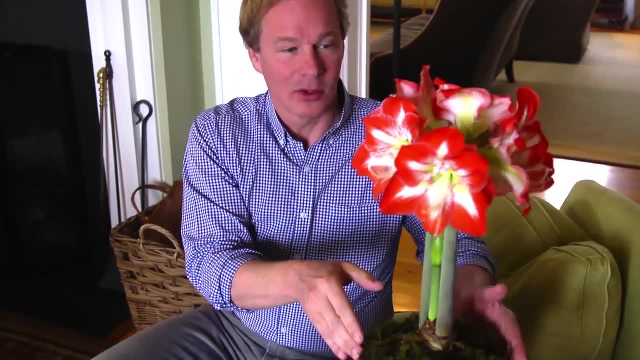 do, These lovely flowers will move in that direction. To keep them centered and straight and not toppling over, you want to rotate the plant once a day, like this. Now, after all the flowers have wilted, you can cut the stems off near the base of the. plant. You see, it's actually this foliage that fortifies the bulb, Such that it will produce another beautiful bloom next year. So when cold weather comes a-calling, have a little fun. Brighten up your house. Plant some amaryllis. 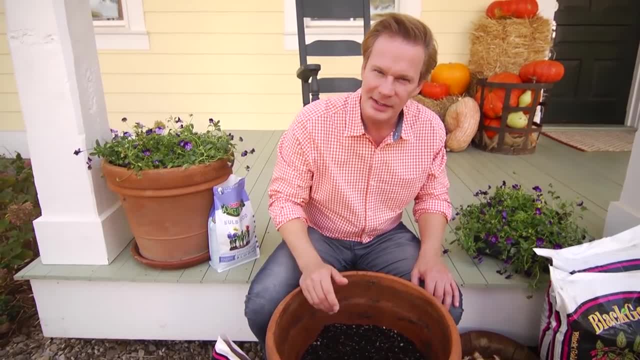 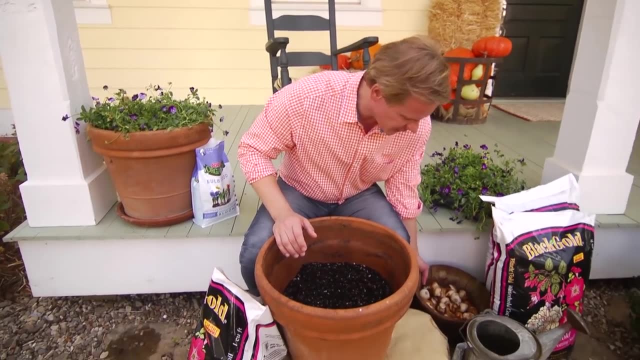 You'll be glad you did. One of my favorite gardening activities in the fall is to plant bulbs. Why, Well, it's so rewarding, It's almost fail-safe. You see, in each one of these tulip bulbs is a flower, already packaged and ready to. 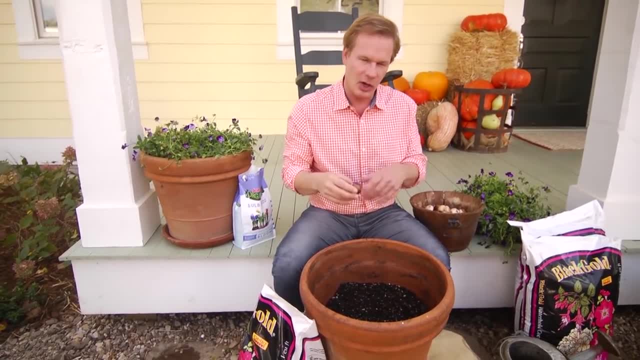 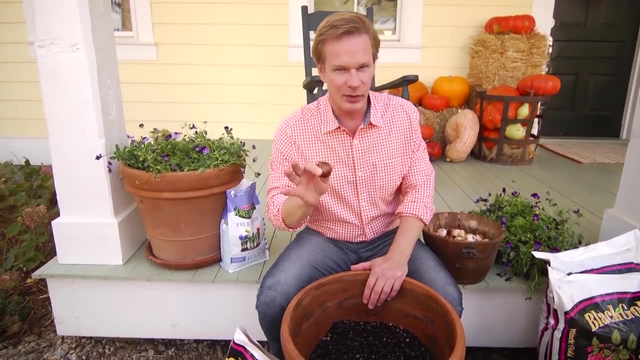 grow. All we have to do is put it in the right environment, Coax it along and, presto, next spring. you wouldn't believe the blooms you'll get Now. the easiest way I have learned to plant bulbs is in a container like this. 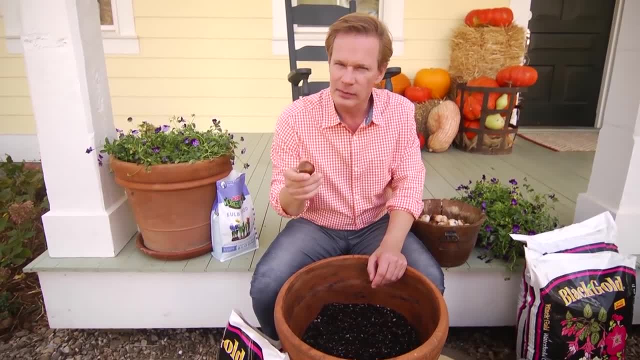 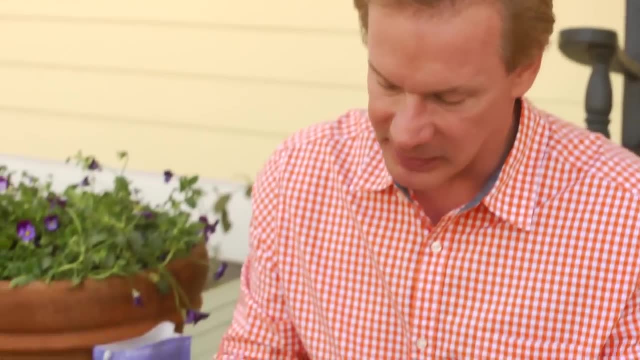 Actually, what you're planting is a bouquet. You see, they're just going to be dormant for a while. Well, I say dormant, they're actually going to be growing, but you won't see them. I take bulbs like this and I plant them in a container about this size. 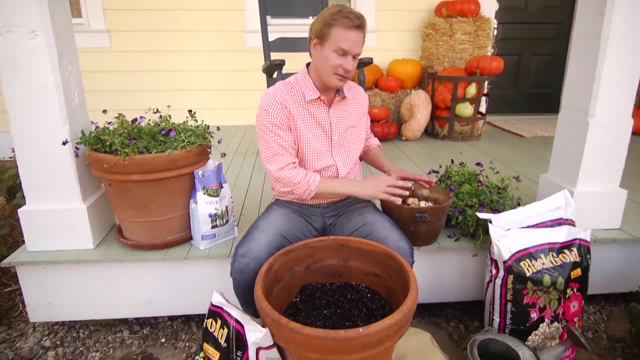 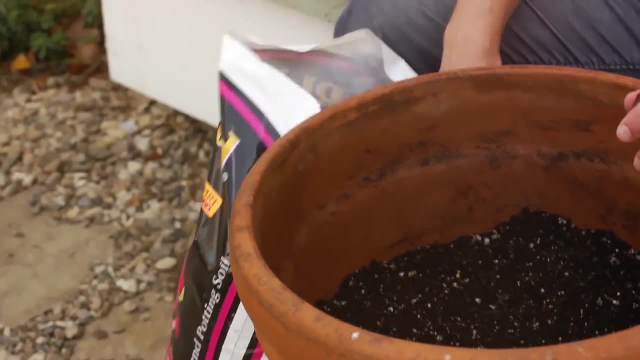 Something that's about a 20 inch diameter terracotta is about right for 50 bulbs. You can see, I filled this up with a good potting soil that's designed for container gardening, So I filled it up about halfway, and then what you want to do is you just want to simply. 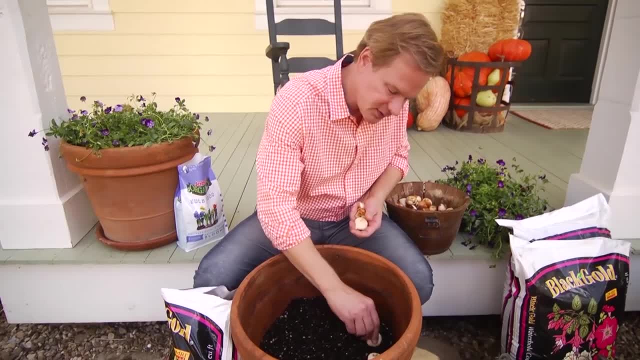 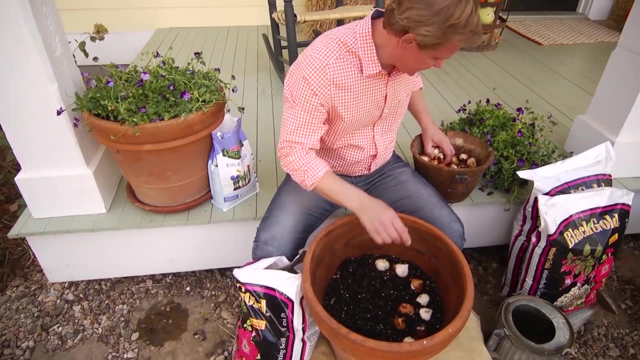 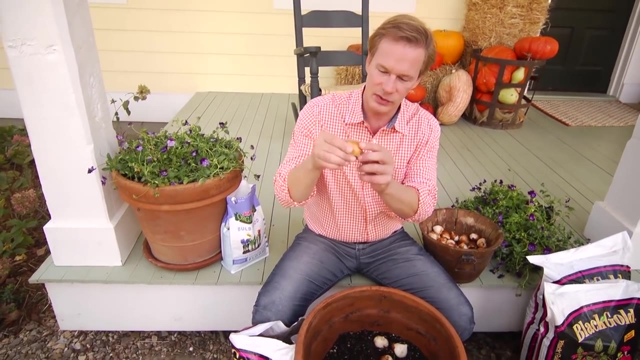 take these tulip bulbs and place them in side by side until this entire basin is filled, just like this. It just takes a few minutes And you want to make sure that you are placing the bulbs with the basal plate this part down. 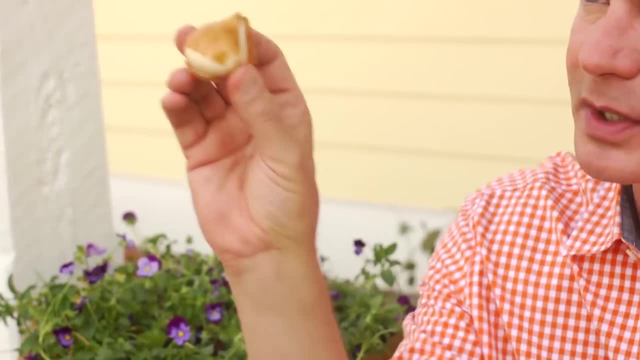 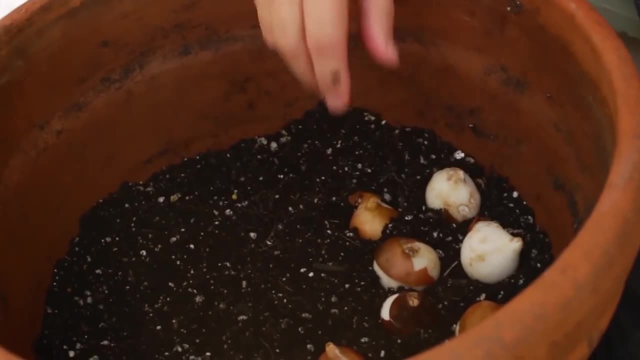 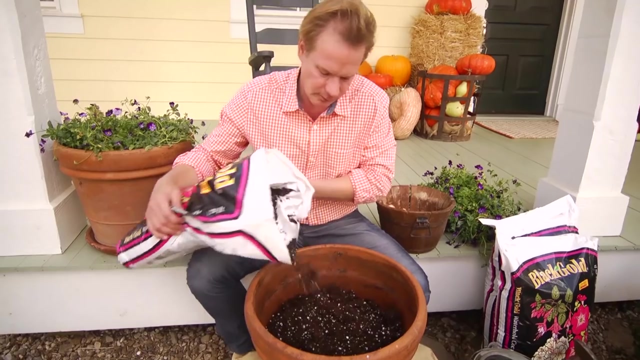 You see, You see the little kiss with the wrapper on it. That's the tunic of the tulip, And the roots come out of that end. the pointy side goes up and you just press them in like that. Alright, now it's time to cover those with about three inches of soil, maybe four. 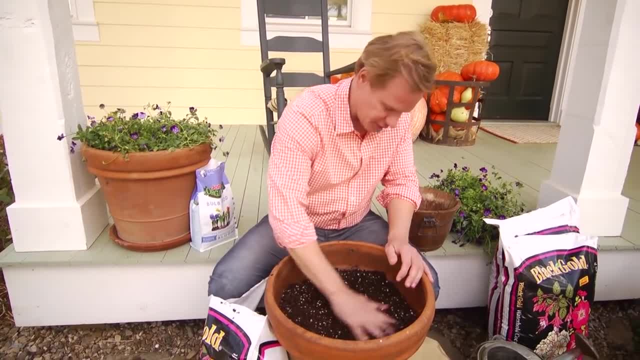 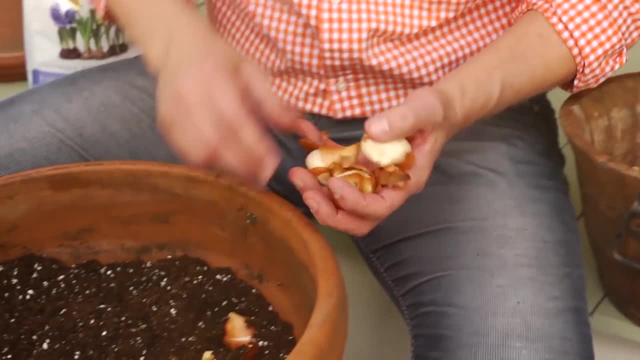 And, believe it or not, you're going to repeat the same procedure. We're going to line another layer up. This is how you get that flower power I was talking about. By the way, this is a great project for kids. they love this. 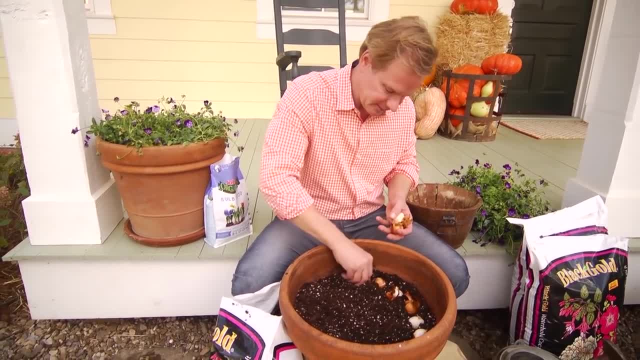 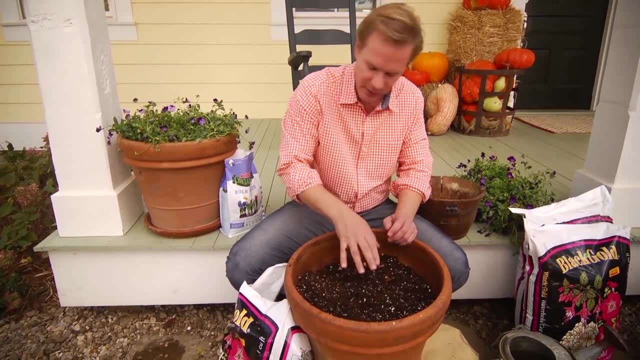 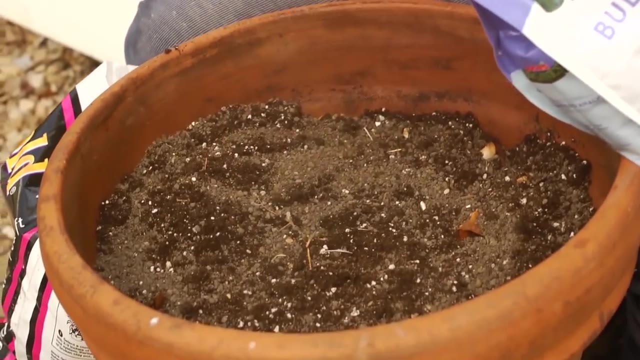 This kid loves it anyway. So next I'm just going to add another little layer of soil here. In the previous layer I had applied about a fourth of a cup to a half a cup of bulb food. I like to use an organic bulb food. 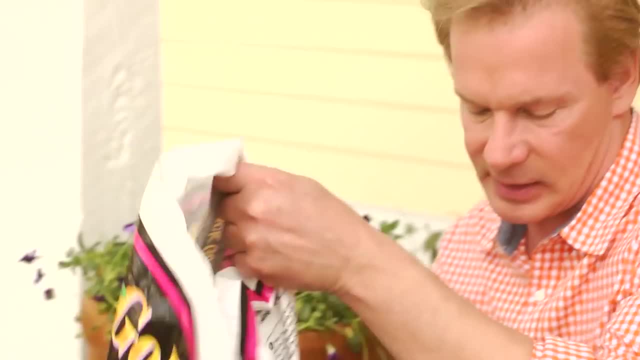 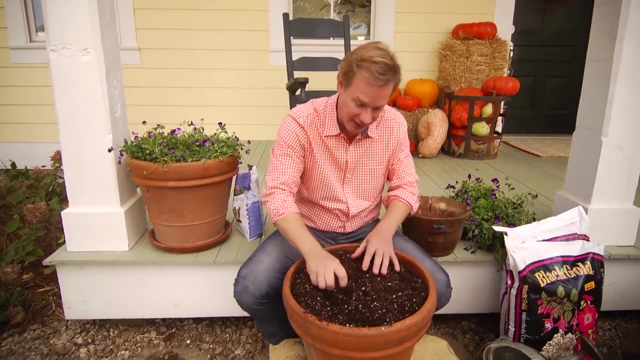 So that'll feed those. And now I'm going to add a little more soil, And there we go. That's about it. That's about it Because I want to finish this off Now. you may think: well, what's going to happen with those tulips? they're stacked on top. 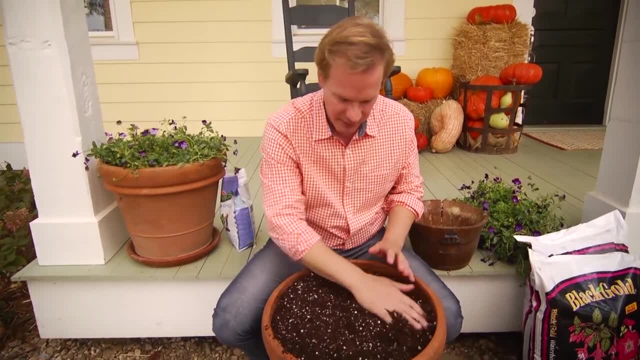 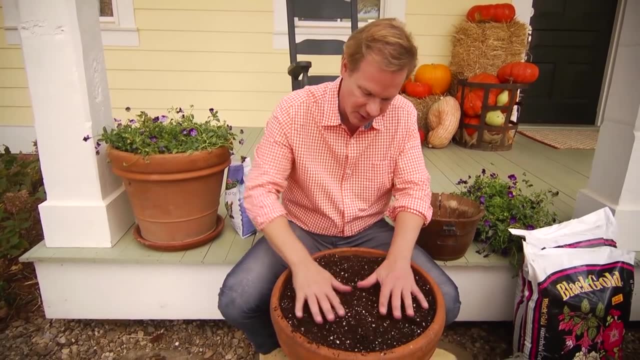 of each other. Well, believe me, Mother Nature has equipped them with the ability they will find their way up around one another over the course of the winter and the early spring. Okay, so I've got soil here on top And I think we can do better than this. 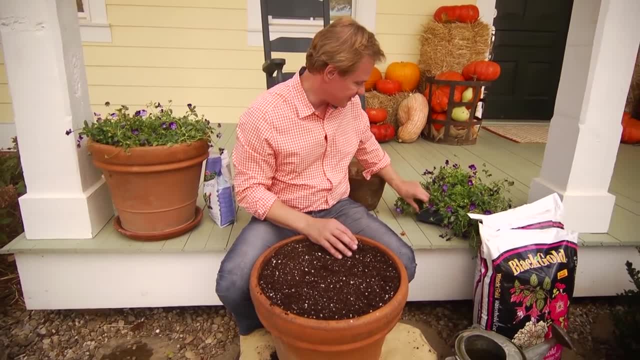 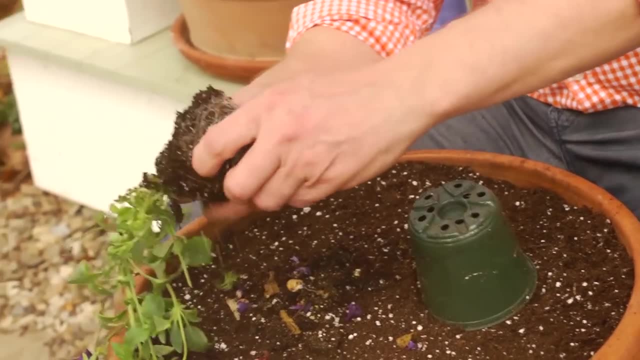 So why don't we over plant it with some of these marvelous pansies? This is a really fun variety. This is a variety of pansy which is one that actually cascades. What I'm going to do is I'm going to just gently tear the roots a little bit and completely 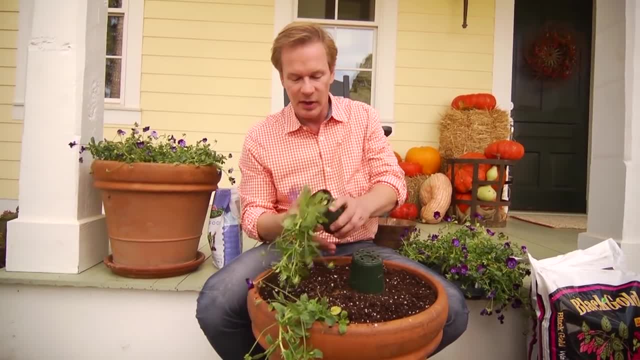 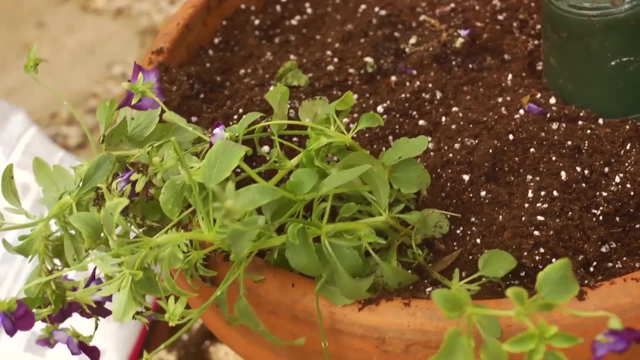 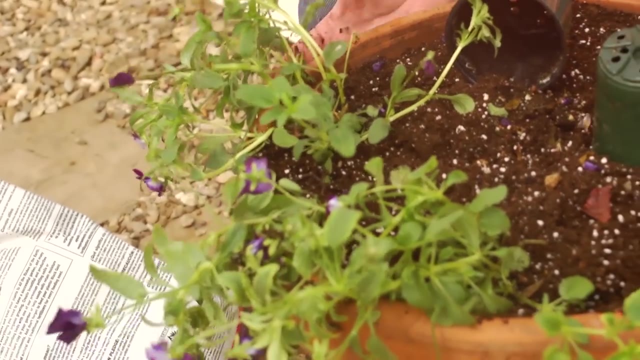 cover this pot. So, yes, the tulips will not only push up between themselves and reach the sun, they will also push up between these pansies. What I love about this particular variety is it actually cascades. So it's perfect for a container like this, because they'll spill over the edge.